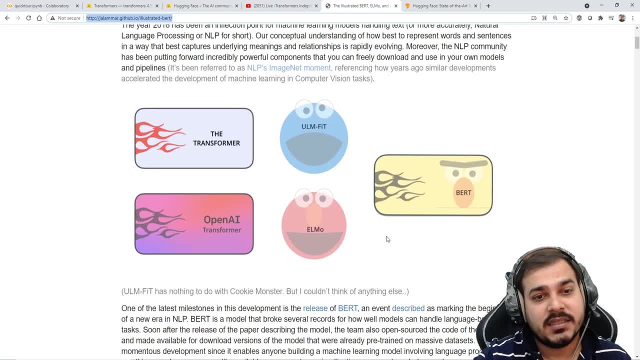 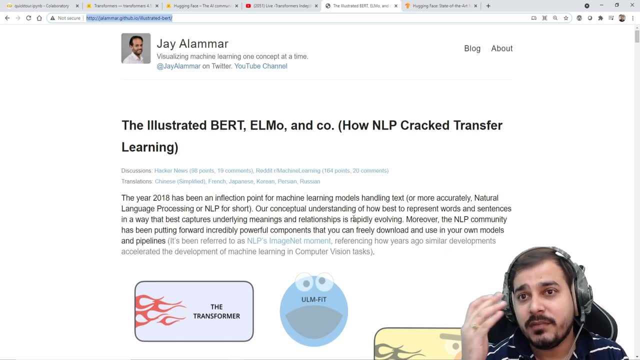 article or blog by Jay Alamar and he has explained it properly, amazingly right. What we will focus on doing: the implementation part. So every day we'll try to do some different kind of implementation and for entirely for this particular implementation, we are going to use Hugging Face. 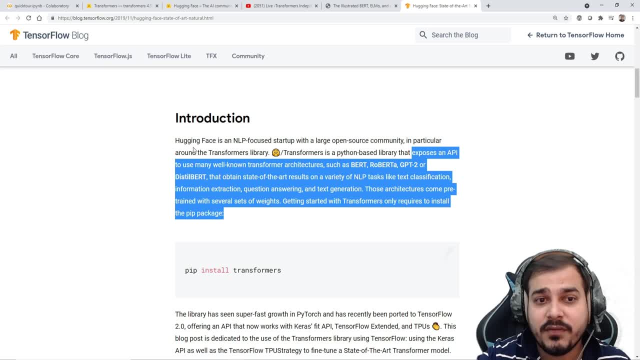 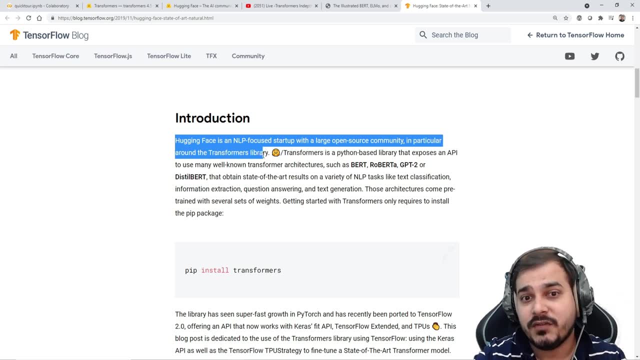 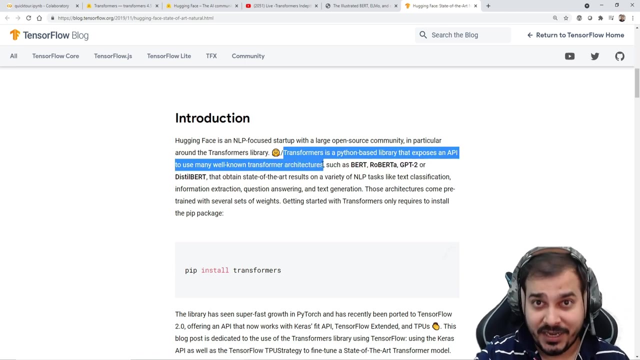 Libraries, Transformers. So over here, what is Hugging Face? See guys. Hugging Face is the NLP focused startup with a large open source community, And particularly around the Transformer library. So Transformer is a Python based library that exposes an API to many well-known Transformer architecture, such as BERT, Robota, GPT-2 or 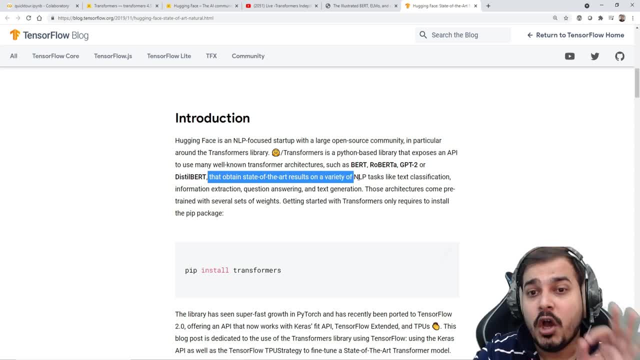 Distilbert that obtains the state of art results on variety of NLP tasks like classification, information extraction, question answering and test generation. So this particular library that is Transformer- it has a lot of state of art algorithms which we can actually use as a 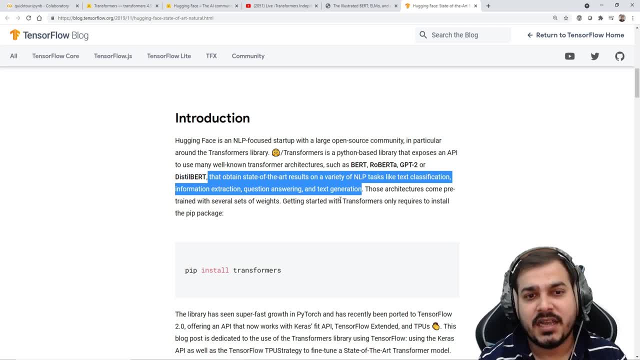 learning technique for solving most of our NLP use cases, like test classification, question answering session, probably masking test generation text summarization. There are many, many tasks And then we will try to see all these things, And tomorrow probably, if you have a new use case where 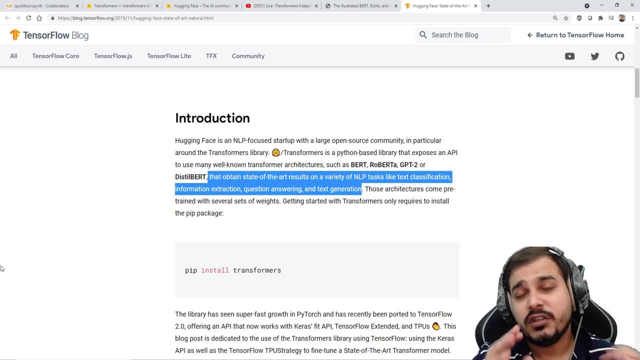 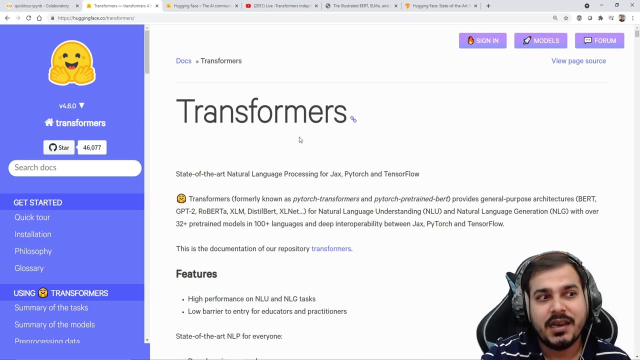 you want to implement some NLP tasks for your company, you can also use this particular library as a transfer learning technique, and then you can fine tune and you can train your model based on your specific data set. So this is the basic implementation with respect to Transformers, And here I'm just going to use Google. 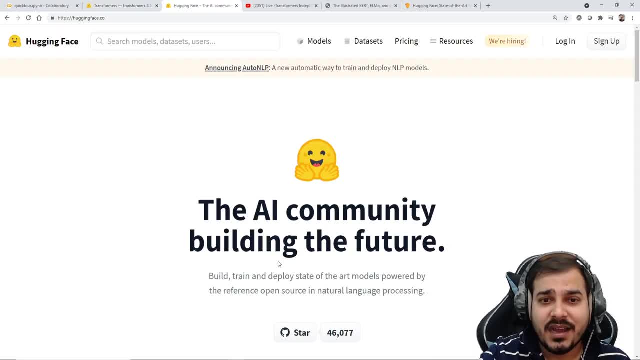 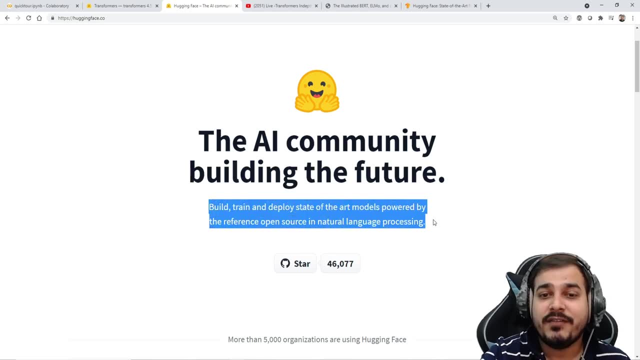 Collab Pro. You can also use Google Collab. This is the hugging face. It is nothing but the AI community building the future. Build, train and deploy state of art models powered by the reference open source in natural language processing. So many companies use this, like Facebook AI, Google AI. 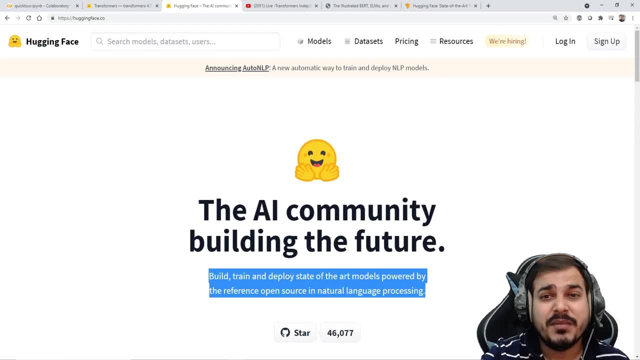 Microsoft, SpeechBrain, Amazon and a lot of examples. A lot of amazing, amazing things are actually there, And they have also come up with this recent auto NLP, which actually helps you to train and deploy the NLP models. So let's begin, And again, this entire playlist is going to be very 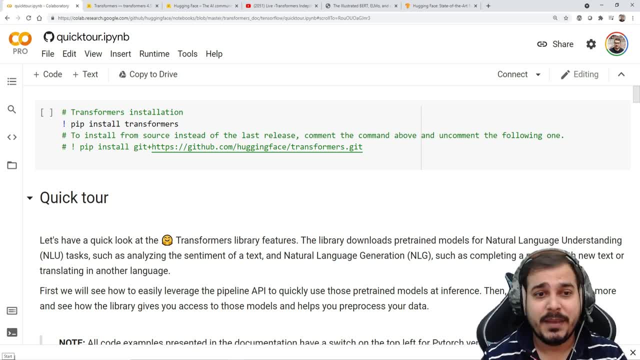 very big, So you'll be learning many things along with me, And probably I've also not learned it completely to a step, but this will give me an opportunity to learn and then probably upload a video. So let's go ahead. I'll just go in to connect to my runtime. First of all, let's change the runtime. I'm just going to. 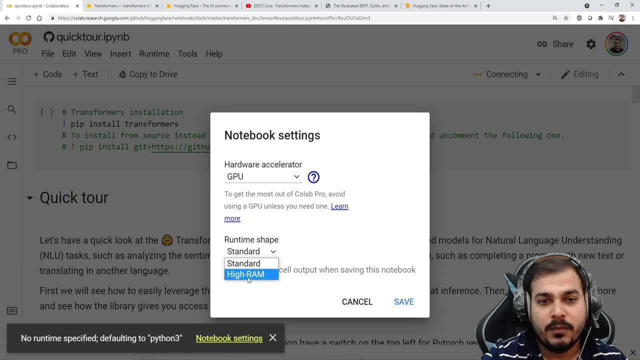 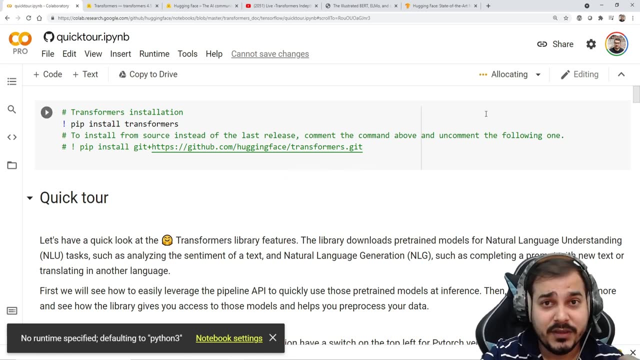 make it as GPU, Okay, And probably I want high RAM because I'm using Google Collab Pro- Okay, So this will get initialized and let's start. how we are, We'll basically start. What are the main things with respect to transformers, How it is able to do all this kind of task, will try to understand, But today we'll just 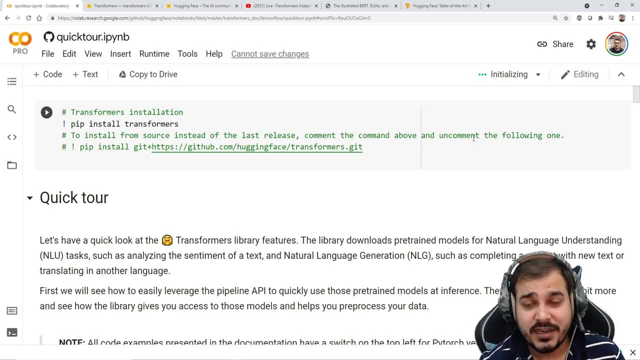 try to see the power of transformers. Different different tasks will try to see what transformers can actually solve. So let's go. So the runtime is ready. Now I am first of all going to pip install transformers. This is how you have to do the installation with respect to transformers. 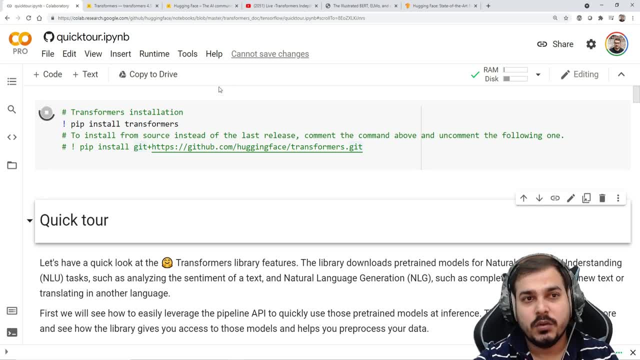 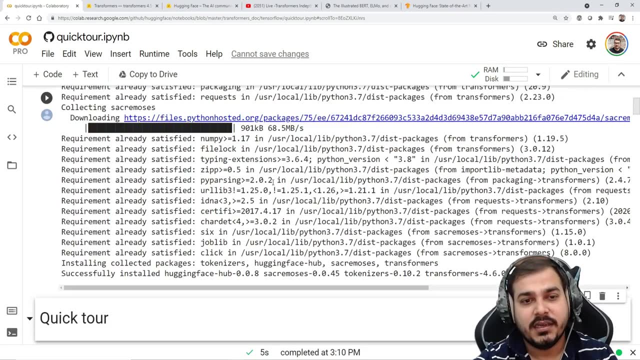 So I'll just execute it. So I'll give you this entire Google Collab Notebook, probably in the description. You can definitely check it out, Okay, So now you can see, the requirement is getting installed Right. So transformers is there. You can either also install like this, or you can also install just by writing: pip install. 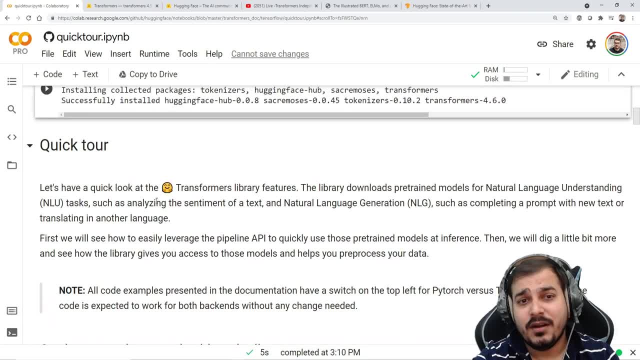 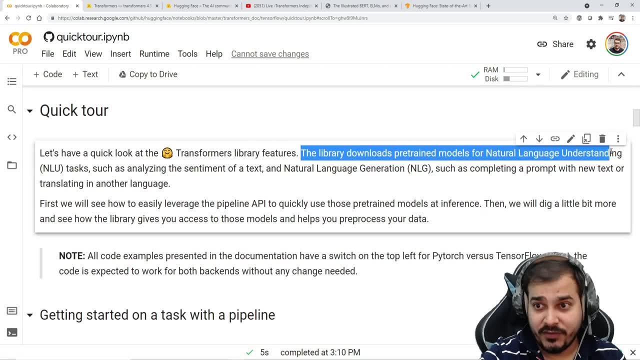 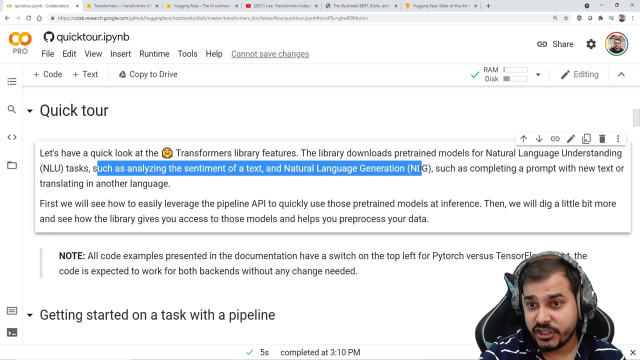 transformers. Okay, Now let's understand what transformers are good at. what transformer libraries are good at. Okay, The library downloads pre-trained models for natural language understanding. That is NLU task, such as analyzing the sentiments of a text, natural language generation, such as completion or prompt with new. 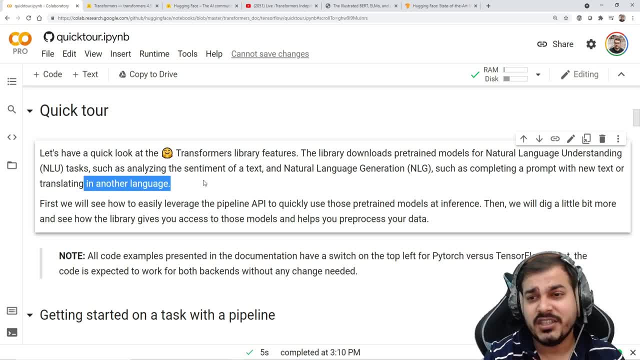 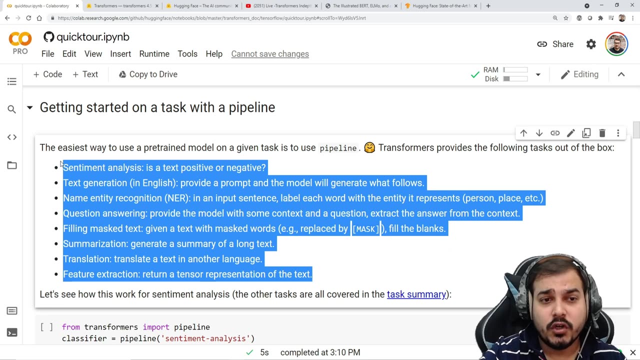 text or translating into another language, So translation is also there. Sentiment analysis is also there, Completing a sentence is also there, So sentence generation is also there, and there are many things. So let's start how this can be done And some of the use cases that have been mentioned over here. Okay, So the easiest way to use a pre-trained 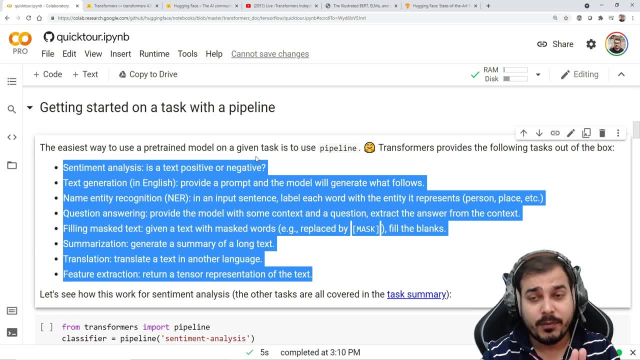 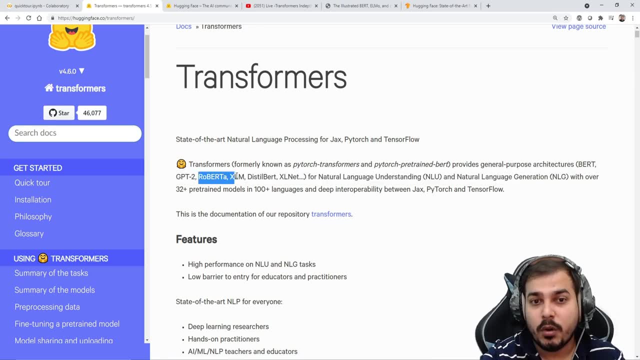 model. So this transformer has a lot of pre-trained models that are developed on BERT architecture. Okay, So if I go and see over here see what all general purpose architecture it has, BERT GPT-2, Robota. 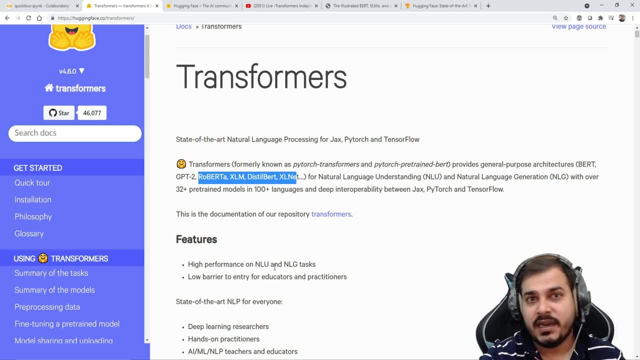 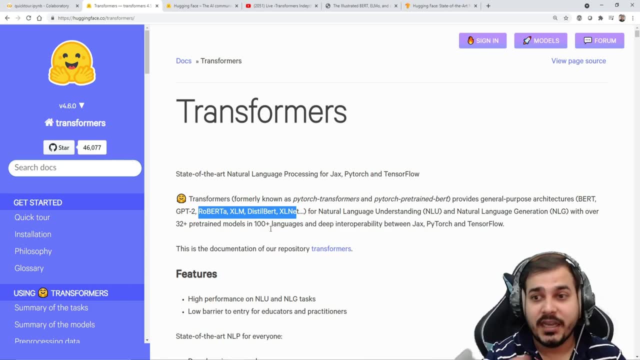 XLM, digital BERT, XLNet. you know all these things are there and we'll focus on implementation of this kind of BERT Whenever the architecture is basically required. I will show you the architecture when we are using this. Okay, So, to begin with, what we are going to: 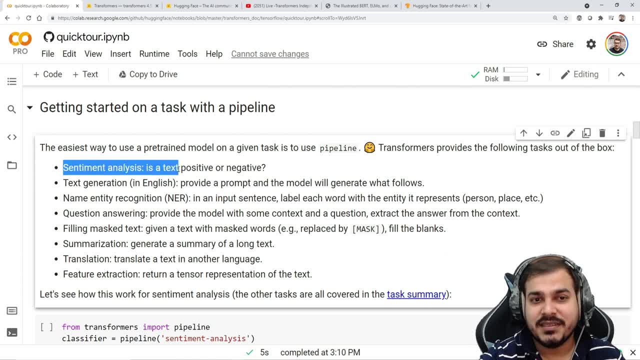 do see over here some of the use cases that has been mentioned, like sentiment analysis, whether a text is positive or negative, text generation, English right Name entity Cognition, question answering, field masters, summarization, translation, feature extraction. Okay, Now see how this thing is implemented and how. 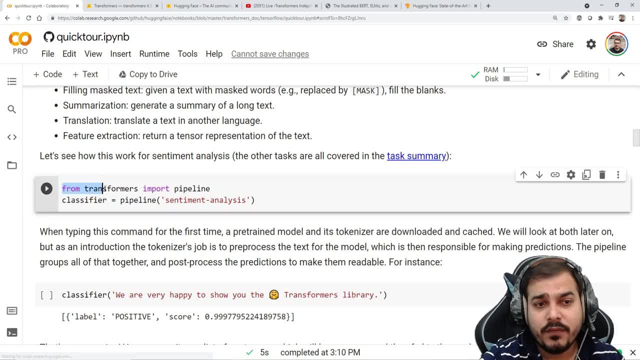 simple, it is Okay. So over here, first of all, you import from transformers. you import pipeline. Whenever you import pipeline, guys, two things gets loaded: Okay, Whenever you're using this pipeline. Okay, So here probably they should be giving something regarding pipeline. 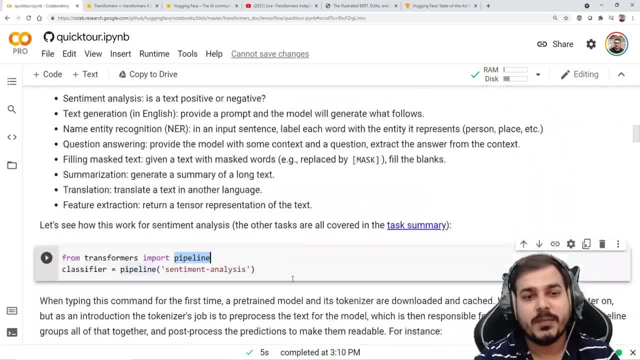 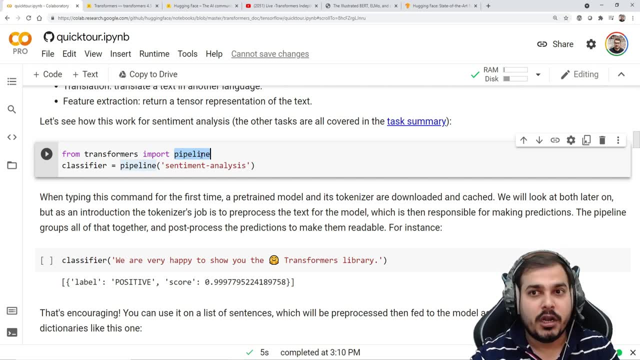 I guess. If not, it's okay, Not a problem. Let's let me explain what this exactly does. Now, this pipeline helps me to call a pre-trained model. Okay, That pre-trained model, maybe with respect to a BERT architecture, maybe with respect to a digital BERT. it may be a GPT-2.. 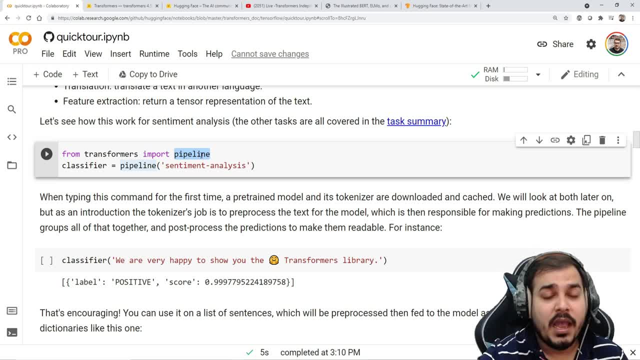 So different types of pre-trained models will be able to call, and that pre-trained model has to be called with this pipeline library. Okay, So here you can see. once I import this, I just have to write pipeline, and I just have to give my one example of sentiment analysis. 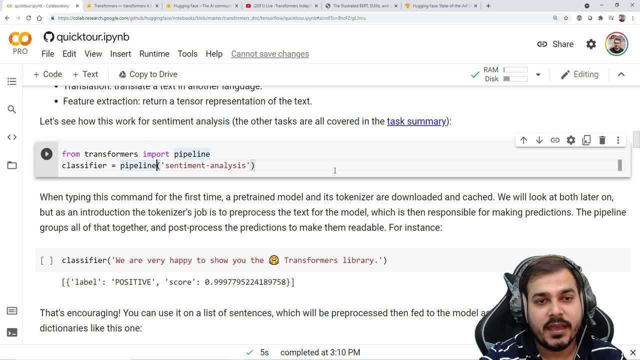 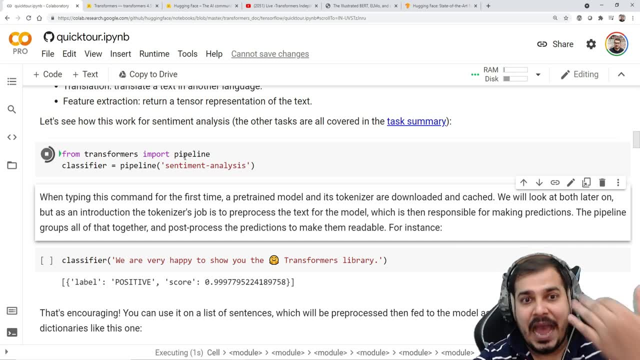 So this is basically a use case sentiment analysis. So if I probably just execute this Okay, I'll show you. Okay. So this sentiment analysis, now what, what happens in the backend? I'll just talk about it, And probably this will take some time for this particular model to get uploaded. 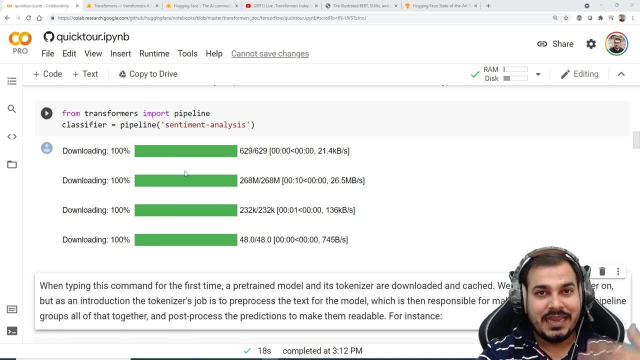 So, guys, once you execute this here, you'll be seeing that that pre-trained model will get downloaded, and it may probably take some time. It depends on your internet speed, right? So right now, this particular model will be focusing on doing sentiment analysis. 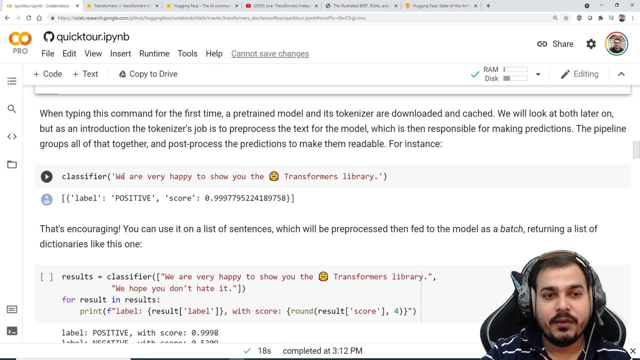 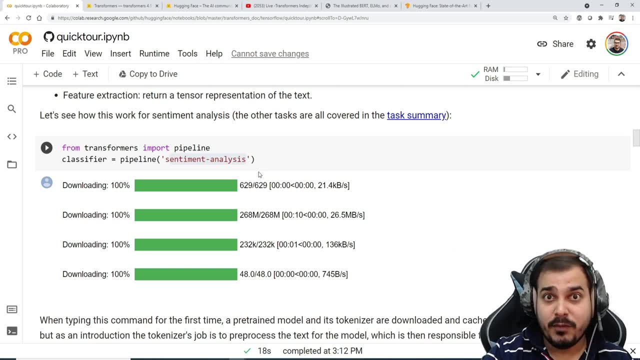 Okay, Now let's see one example. So here we have given like we are, we are happy to show you the transformer library and we are just giving this classifier. And remember, this classifier has a pre-trained model on sentiment analysis. which classifier is getting called? 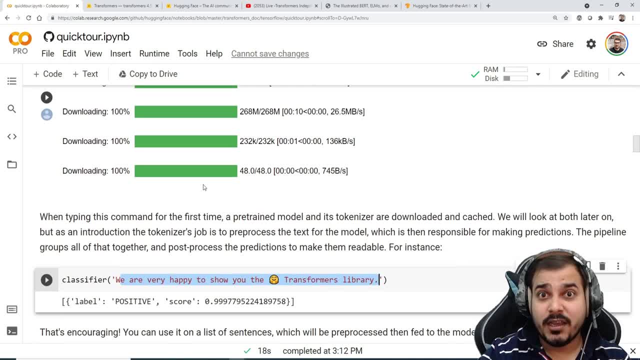 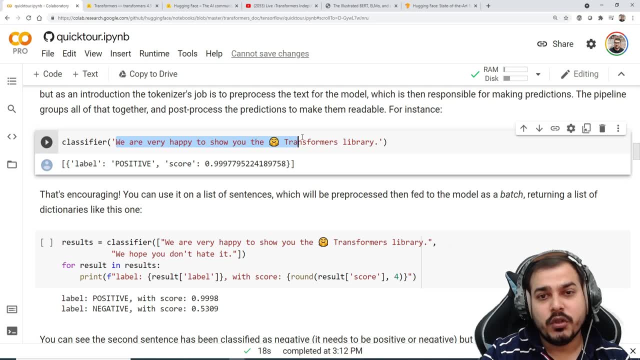 I'll talk about it. Okay, Which classifier or which- probably- model is getting called? which BERT model is getting called? that I'm also going to discuss. Now you can see a way here. I've given a sentence. We are happy to show you the hugging face. transformer library. 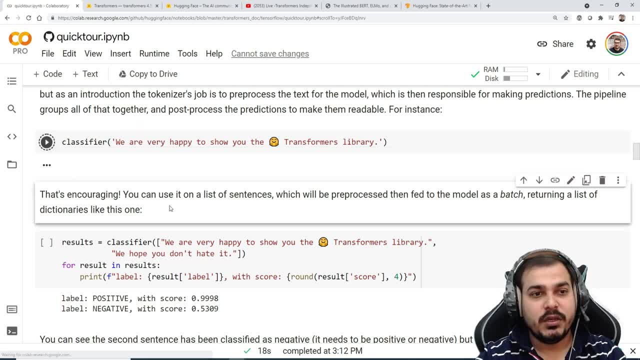 So this symbol is basically of the hugging face. Now, if I go and execute it here, you'll be able to see that I'm getting a positive. It's cool. This also handles well The reason why I'm saying you that. 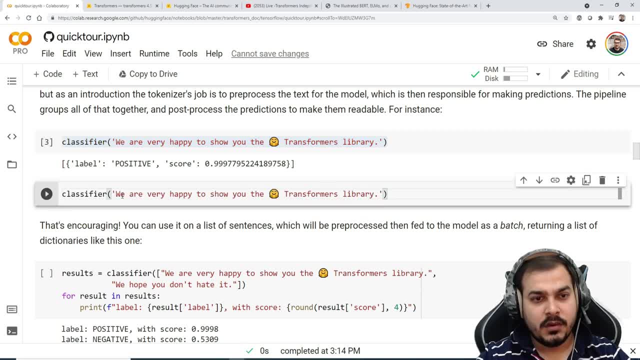 let me just try it over here. I'll just say I don't like pizza. The food is not that great. Okay, Suppose, if I want to execute this here, you'll be getting two values: One is label and one is score. 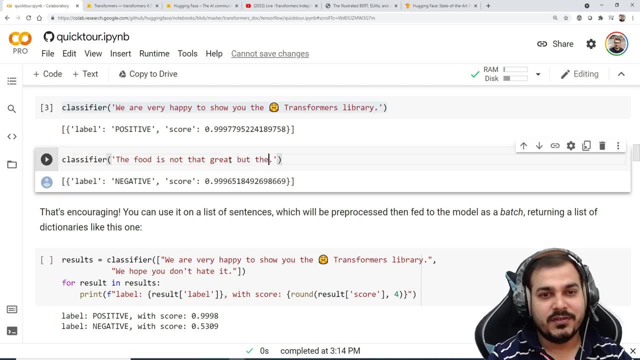 The food is not that great- I can also confuse this, but the crust. the pizza is not that great, but the crust is awesome. Suppose I give you something Like this: The pizza is not that great, but the crust is awesome. 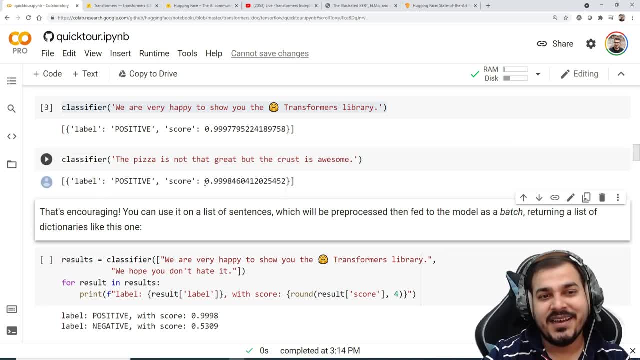 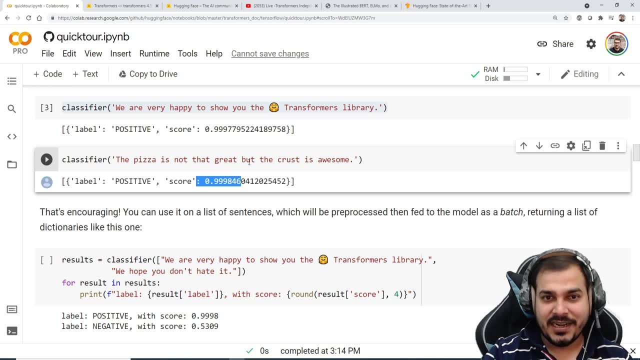 So once I execute it here, you'll be able to see, okay, how this gives us a positive score. But here you can see that, right, It is little bit intermixed, right, The pizza is not that great, but the crust is awesome. 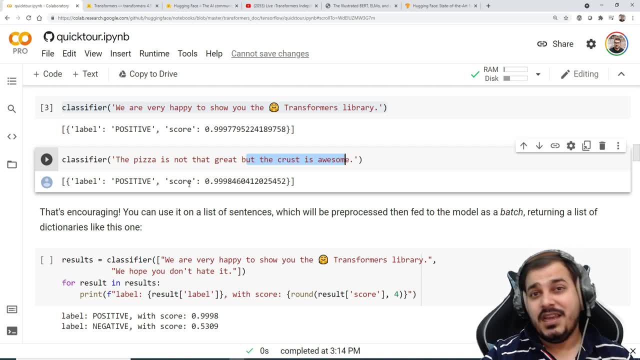 So just by seeing this, probably awesome, I think we are getting a high score. But yes, if you see different, different scenarios there, you'll getting a probability of somewhere like 0.53, 0.54 like that. Okay, 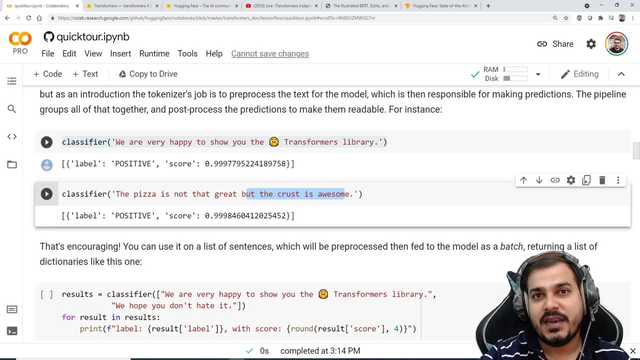 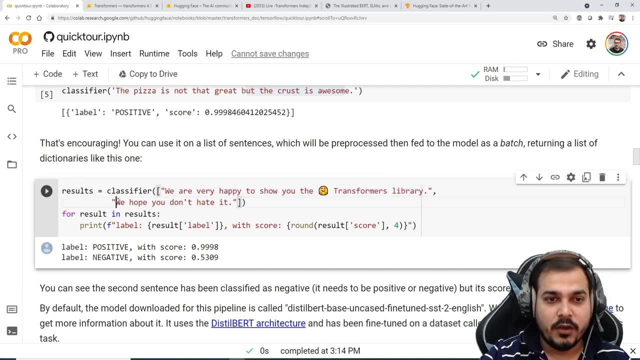 Now let's see, with the help of this specific library also, what you can do. you can also give multiple texts, like how we are given in this. We are happy to show you the transformer library. We hope you don't hate it. 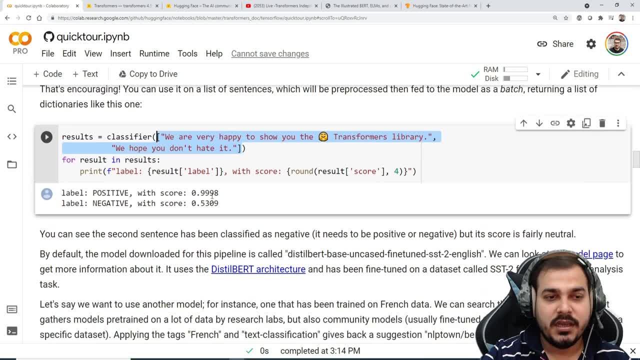 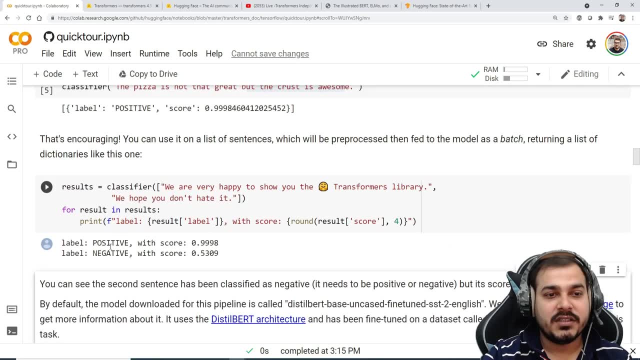 Okay, So two texts are there. Remember you have to give it in the form of list and then you can also check the label and the score. Okay, So I'll just try to execute it over here And here you'll be getting somewhere on. this is positive. 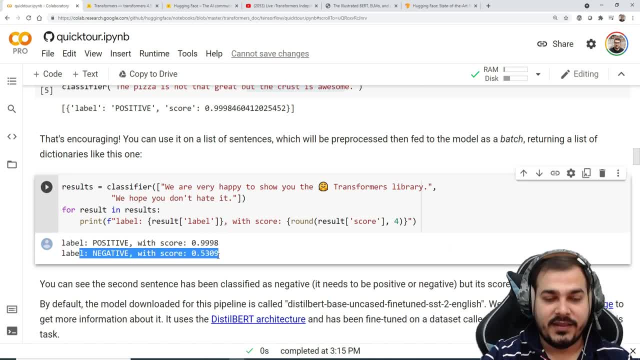 It is 0.99.. And this is negative with score 0.53.. Now see, in this particular scenario- we hope you don't hate it, Right? This is just like a question, not a negative statement, you know. but it is actually giving you a score of 0.53 with negative. 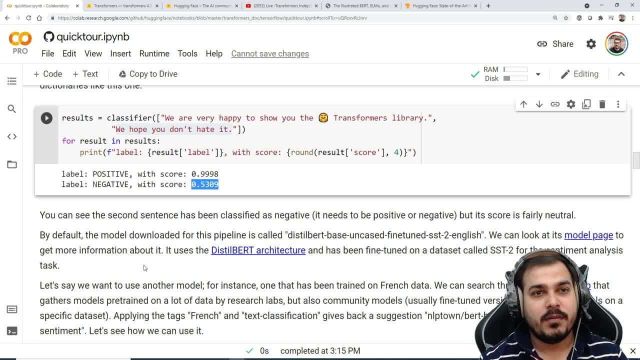 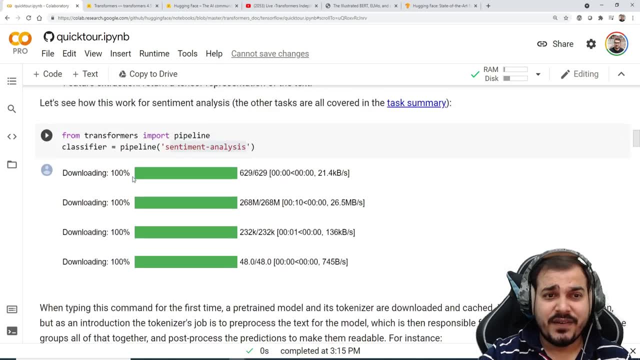 Okay, So it is just like a neutral. You can also classify this probabilities based on different, different categories. Okay, Now, this is very important: When I'm calling this classifier: what exactly is happening, Why the sentiment analysis is able to give this particular 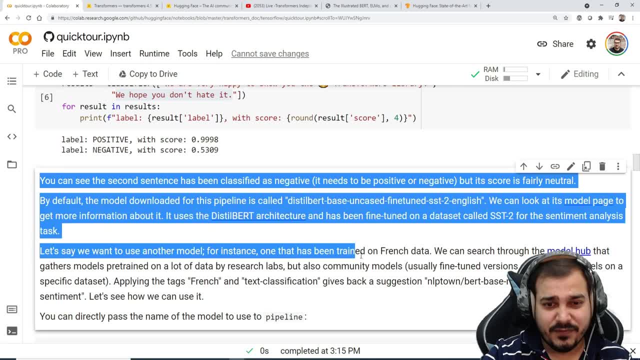 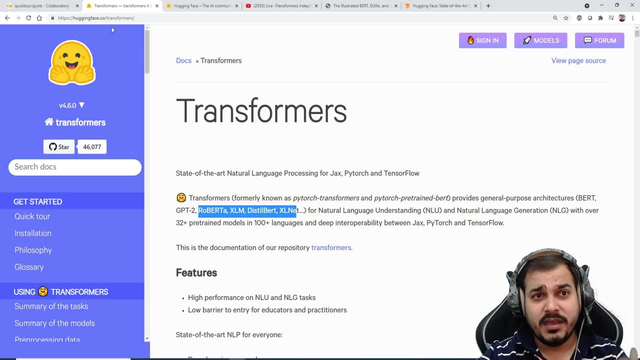 output. we'll try to understand. Okay, Now see this guy. the sentences are very much important. It is very much necessary that you read it line by line If you really want to understand. probably, guys, this documentation that are given with respect to this transformer. 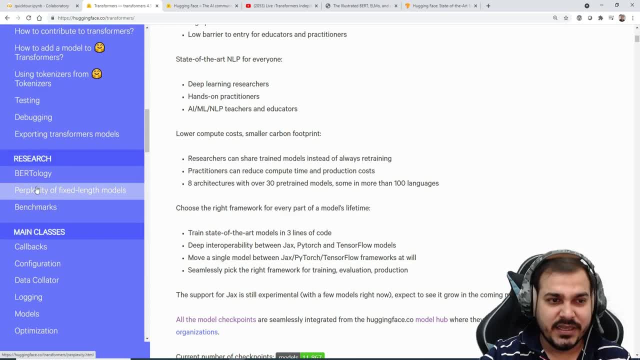 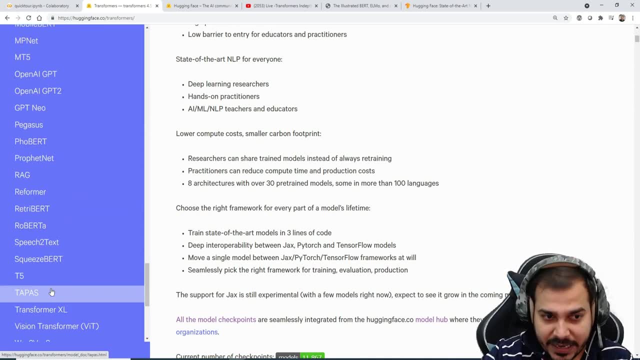 it is pretty much amazing And, trust me, I will cover each and everything, each and every points over here with practical implementation, with, with your own use case. I'll try to cover everything that is present over here And it'll be pretty much awesome. 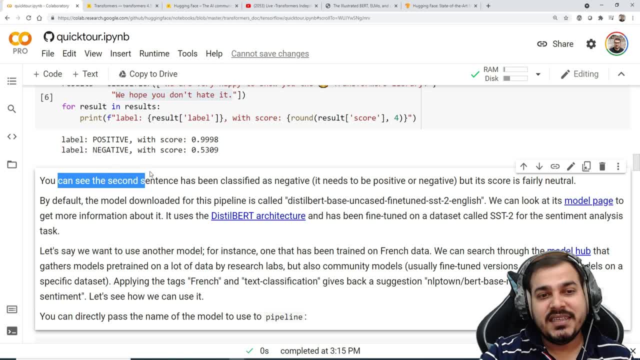 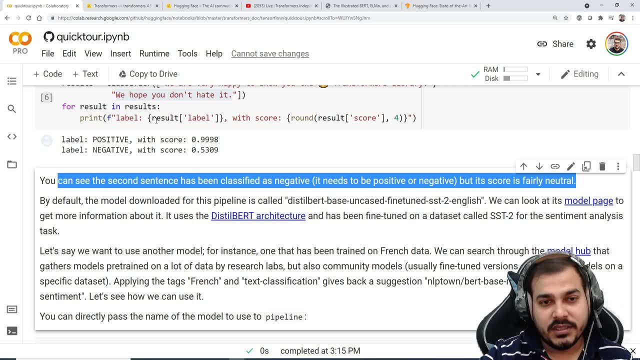 You'll be able to learn a lot of things. Okay, So now you can see. the second sentence has been classified as negative. It needs to be positive or negative, but its score is fairly neutral. Okay, Now, this is the observation that we have made from this particular sentence. 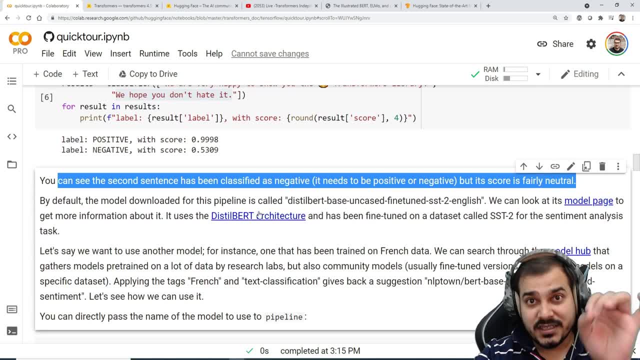 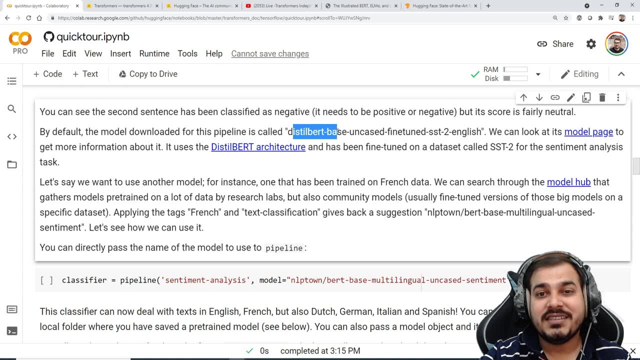 right Now, by default, no model downloaded for this particular pipeline. Now, this sentiment analysis by default, which we have actually downloaded, we have downloaded something called as distal, but uncased, fined, used SST to English right Now why? 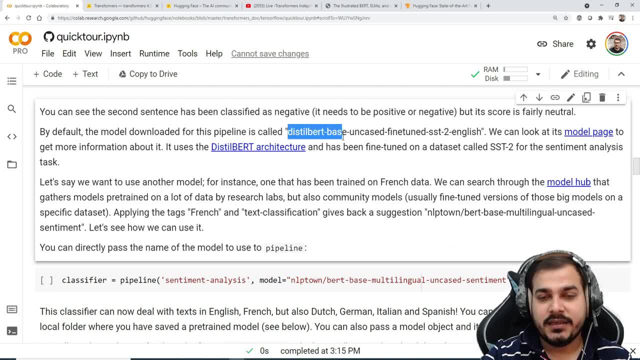 what is all these things, guys? See this, this distal, but base is basically our model, Uncased, basically says that our data set, which is basically trained- right, All trained on small letters. right, All the words are in small letters. 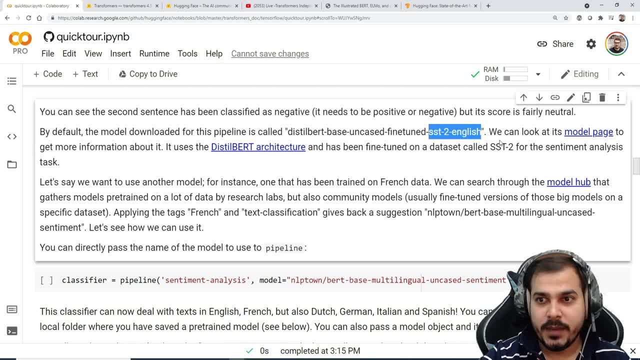 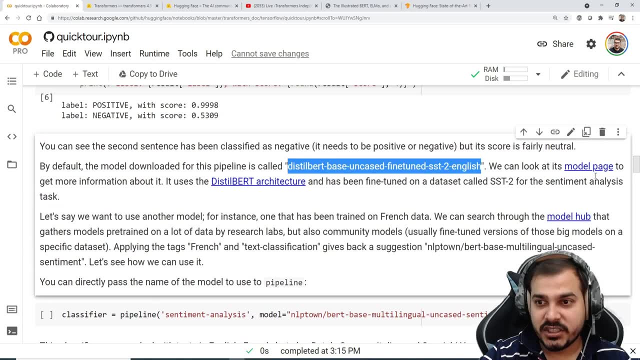 right, And SST to English is basically my data set. Okay, Now, if you really want to find out how many different types of models are there, you can also look out where this particular model is there by just clicking in this link. Okay, 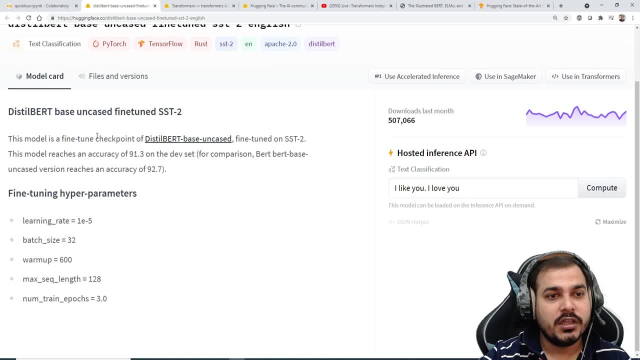 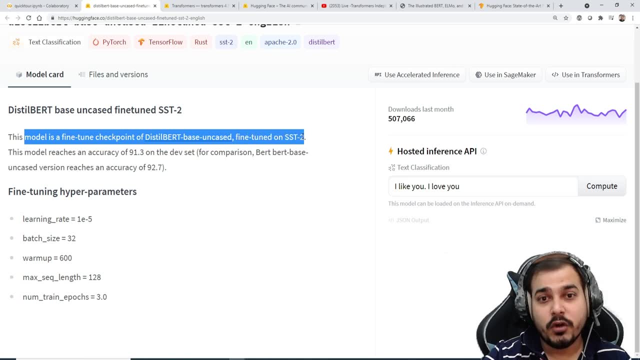 Just go and click on this model page link. here You'll be able to find out all the information regarding this particular model. This model is a fine tuned checkpoint of distal but based on case fine tuned on SST. to that basically, this is basically my data set. 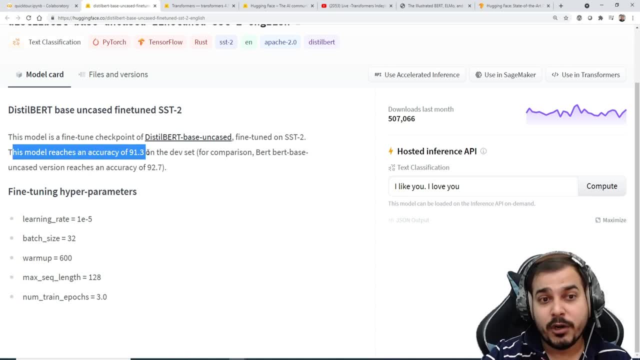 The model reaches an accuracy of 94, 91.3 on the depth set for comparison but, based on case version, reaches 92.7.. So here it is saying that BERT probably performs better than distal BERT. And what are the parameters that are taken in this? 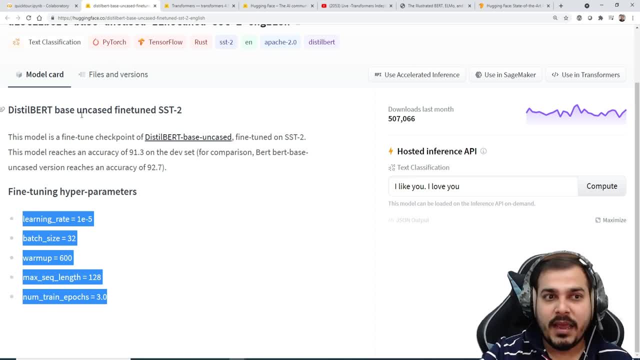 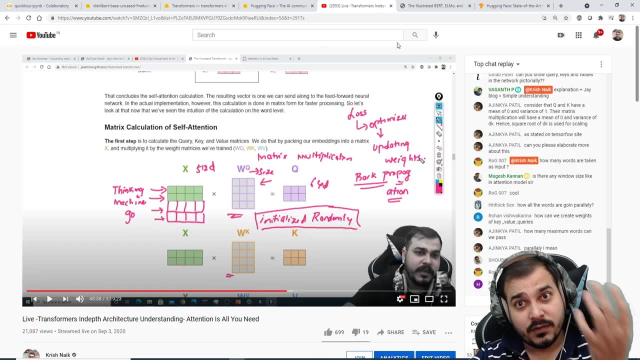 It is somewhere on learning rate, batch size, warm up and all. You'll be able to understand how this architecture works If you know BERT and transformers that always remember that. So I'd suggest just go through my transformer video and really. 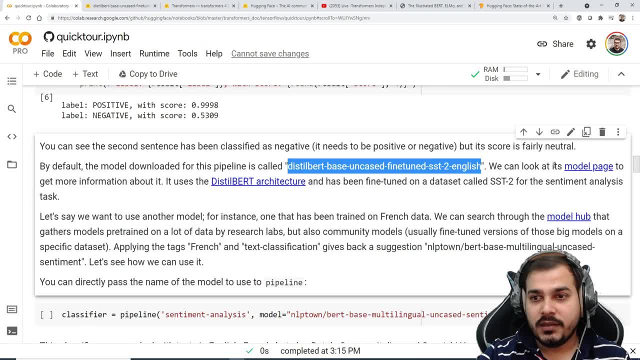 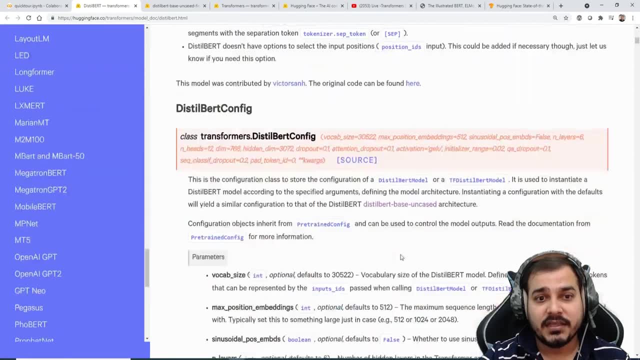 you need to see this particular blog to understand BERT. Okay, Now, this is the information from the model page. If you really want to understand the distal BERT architecture, you can just click over here And this is my entire distal BERT architecture. 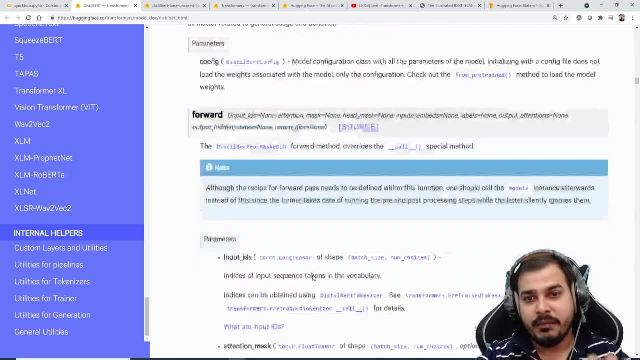 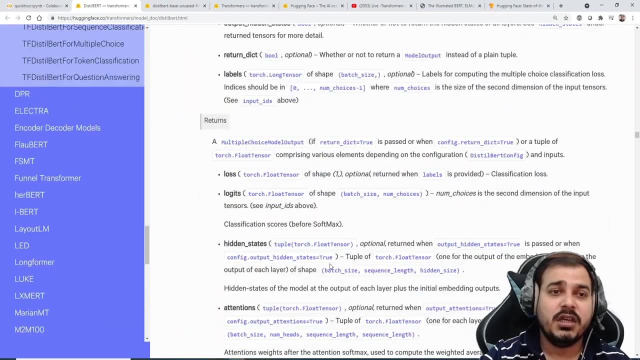 What are things are required? Probably the architecture is not given, but main main things. what are important for this particular architecture is given over here. Okay, And if you really want to find out a distal BERT architecture, always remember. 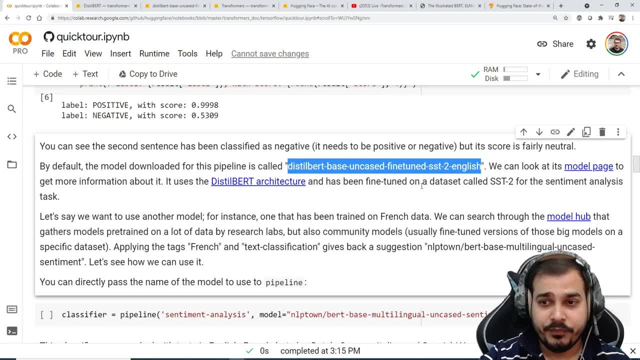 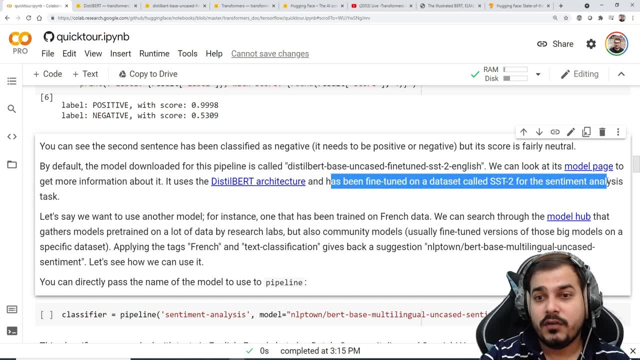 try to Google it and try to find it out. You can also check out the research paper. Okay, Now here you can see. it uses a distal BERT architecture. He has been fine tuned on data set called as S2.. For the sentiment analysis task. 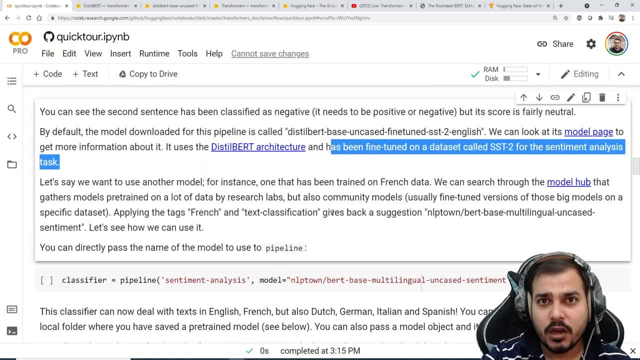 Okay, Now this is fine. Can we call some other model also? Right, Can we call? because in sentiment analysis you'll just not have one model. I showed you right When we were checking, probably this one. let me see when we are checking over here. 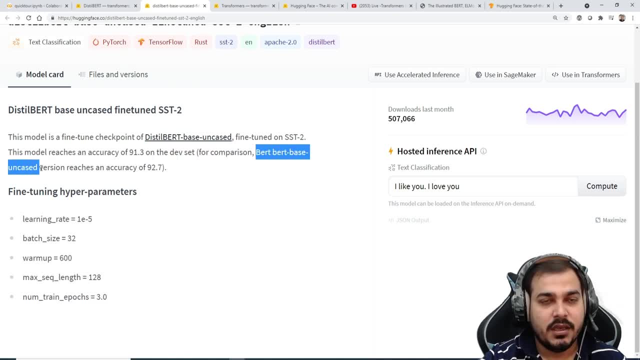 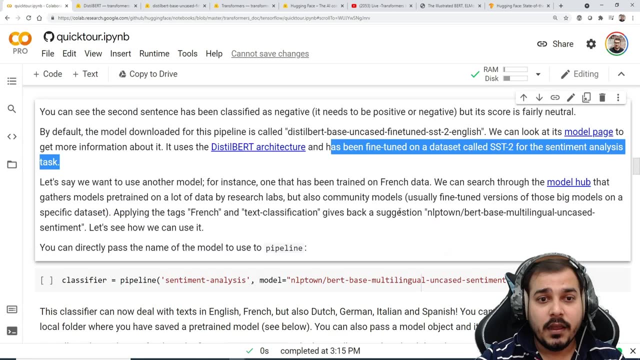 it is also saying there is a model called as BERT BERT base uncased version, right? So with respect to different, different tasks, there are multiple models with different, different accuracy, right? So what I would suggest is that suppose see over here. 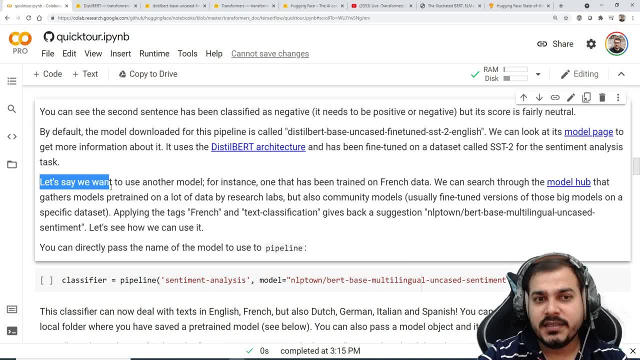 it is given a very nicely, the documentation is given. guys. Let's say we want to use another model, for instance one that has been trained on French data. Suppose I want to work with a model that will be able to do text classification based on French data. 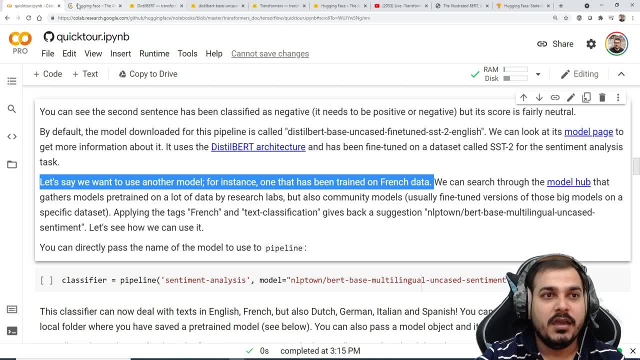 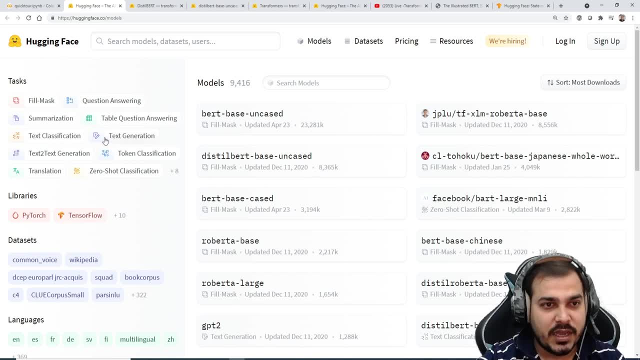 Then we can search that specific model from this model hub. Now, model hub is basically the hub of the entire hugging face models, right For a specific cost. Now suppose I want to do text classification. Okay, Now in this test classification. 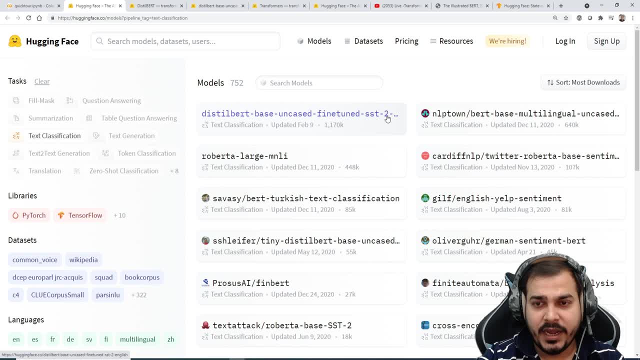 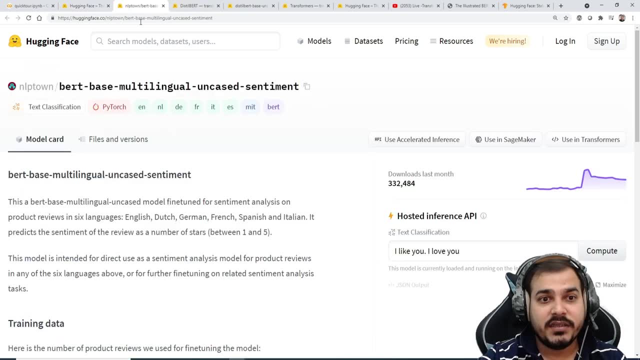 we have applied distal burst, uncased, fine tune SST two right Now. suppose I want to do it for multiple languages. Then I can go and select this NLP town bird based multilingual, uncased, If I go and select this here. 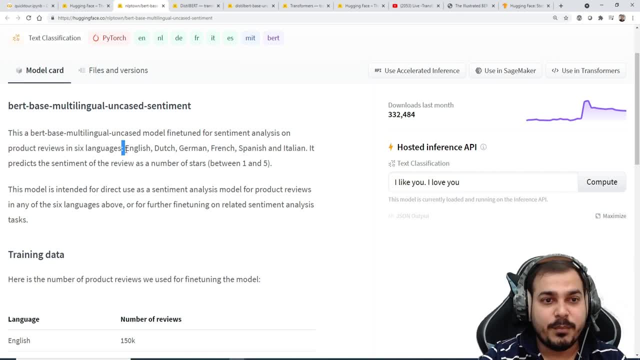 it will tell you that what all languages it actually supports. It's supposed English, Dutch, German, French, Spanish and Italy, Italy. Now, my use case was that I had to use a French tech, Suppose if I'm giving a French state. 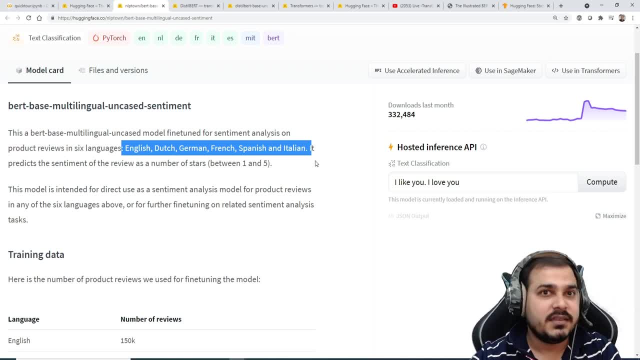 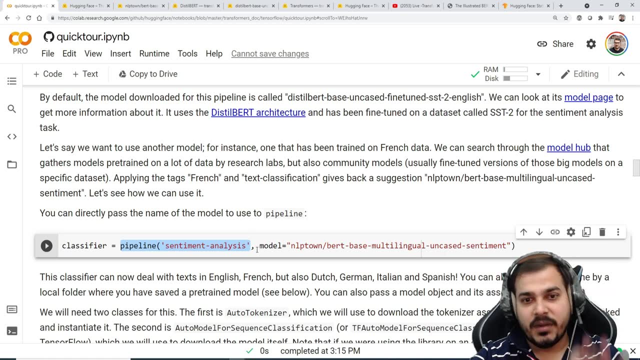 it should be able to crack classify whether the sentence is positive or negative. right, So now what I'll do? I'll again call this pipeline, I'll give sentiment analysis, but here I have an additional parameter. See if I go and see over here. 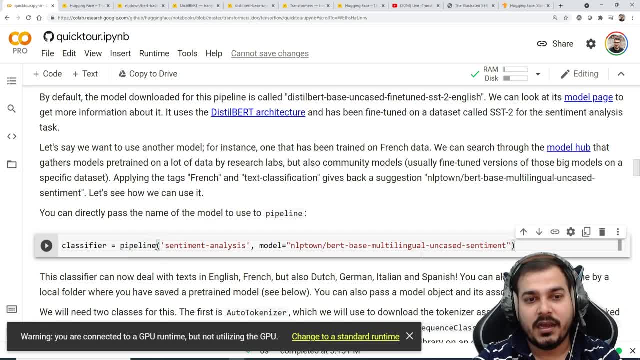 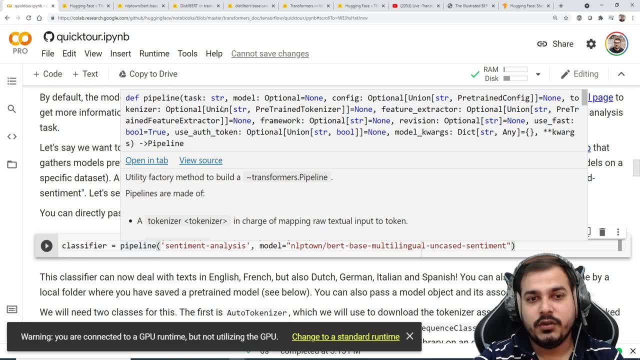 over here you will be able to see the first second parameter that is present inside pipeline. You know, somewhere you'll be seeing model. So model is my second parameter, right, You see? you can see it over here. This is basically my model. 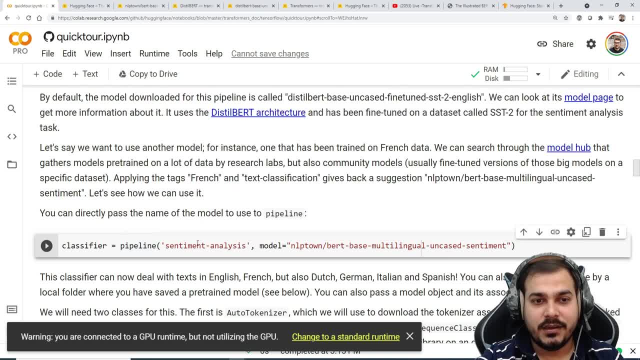 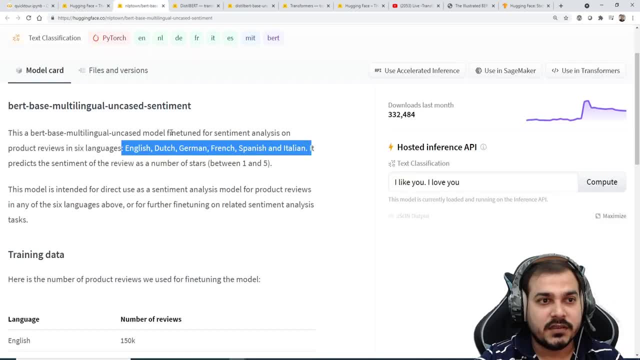 right, It is optional, by default. It takes, uh, the distal, but a model. now, in order to just specify the model, you just have to copy this path. See this, You just have to copy this NLP town, but this entire path. 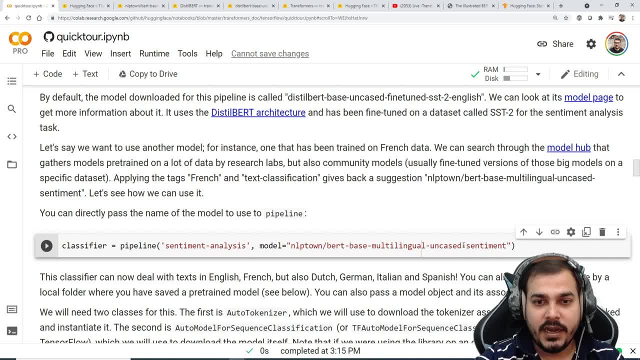 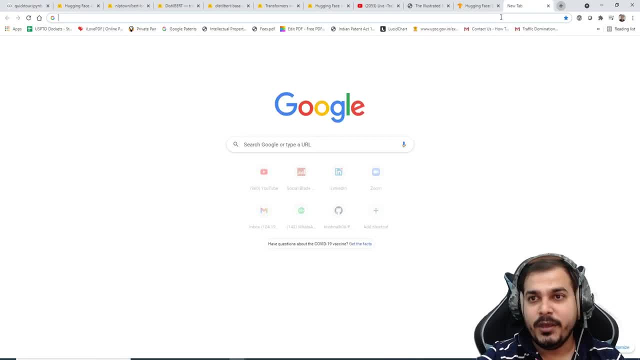 you just have to copy it and you just have to paste it over here, right Once you paste it, now download it. Okay, Now download it. Probably it will take some time for downloading again. Till then, let me open Google translate. Google translate. 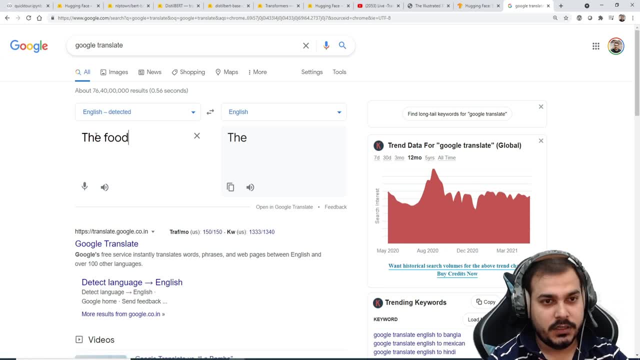 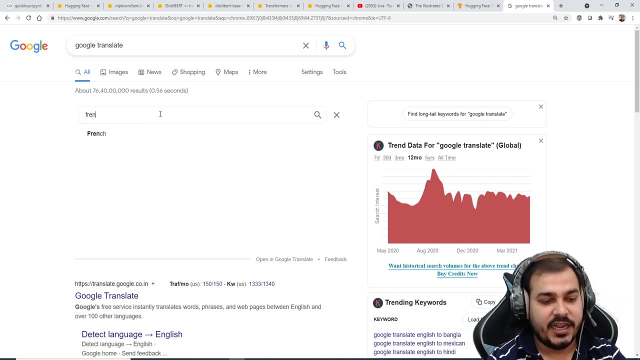 Okay, Now what I'll do? I'll say the food is bad, Okay, And probably I'll convert this into French because it supports French Italian. So I just want to check it. Okay Now, this is my text. Now let's see. 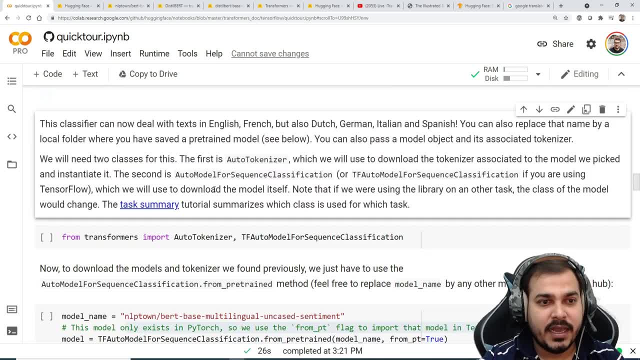 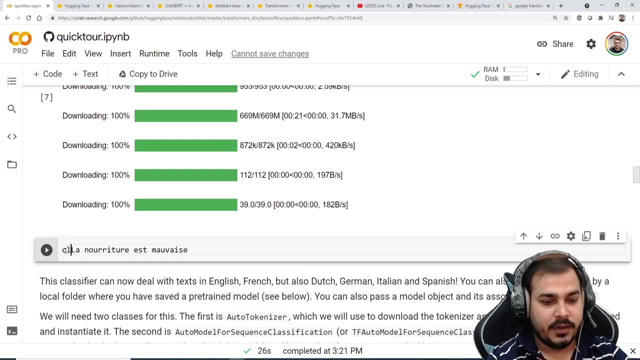 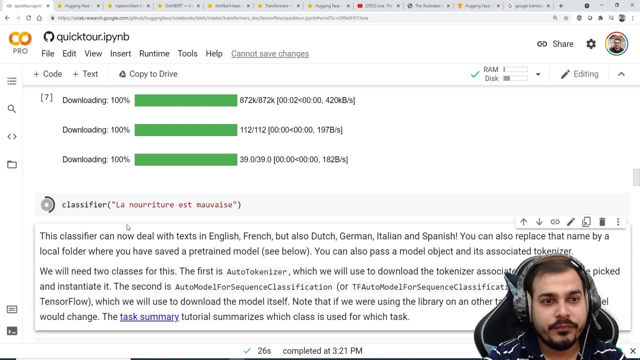 I will just try to execute it over here, So probably this will take some time. Yes, The execution is done. Now I'm going to create a code and probably paste it over here inside my classifier Now, once I execute it here, 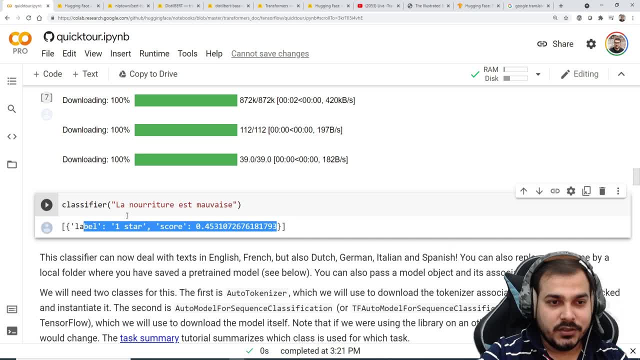 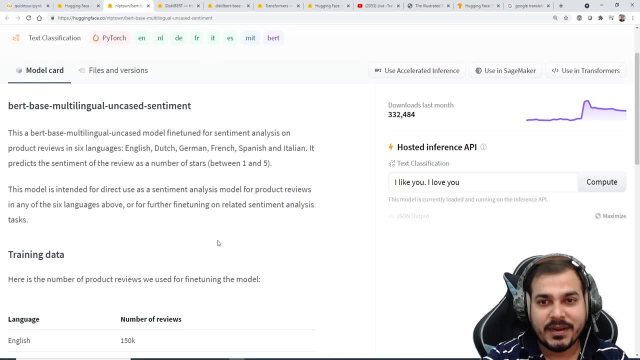 you'll be able to see label start score. This is them. Usually, the outputs Over here is basically given on stars, And for that I really have to check out this particular model, how this thing is given. Now see in this: 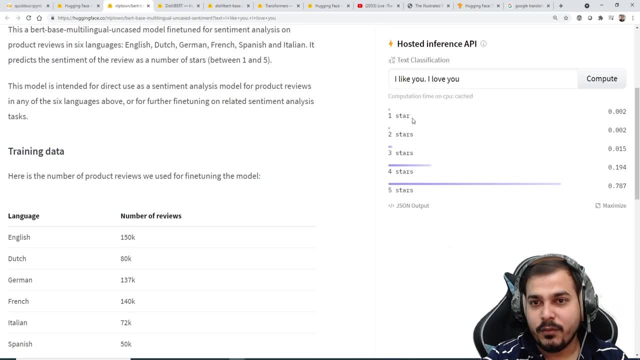 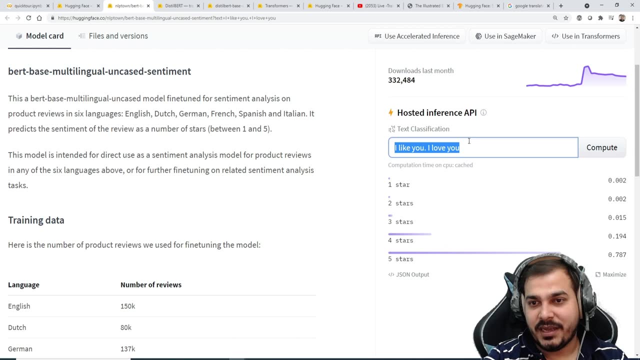 the text classification. if I compute it here, you'll be getting one start to start: three star, four star, five star. Yeah, this is a very, very positive sentiment analysis. So it is saying five star. Let me copy and paste this. 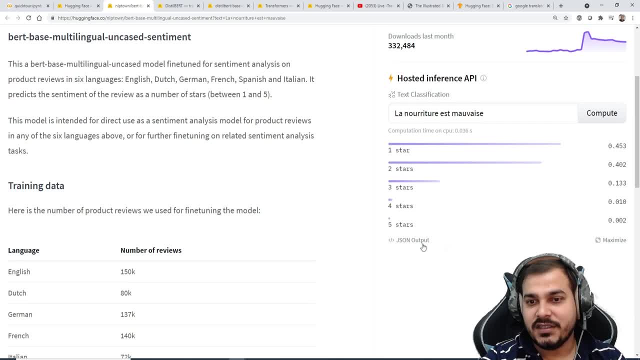 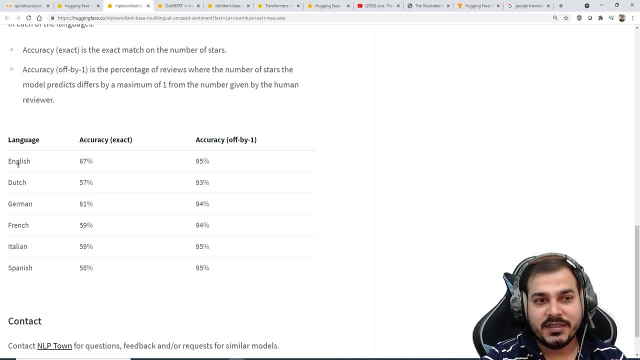 It is also going to give me one star of 0.453,, two star of this, three star of this. So these are all the information that is basically given right? So, uh, what are the accuracy with respect to English language? 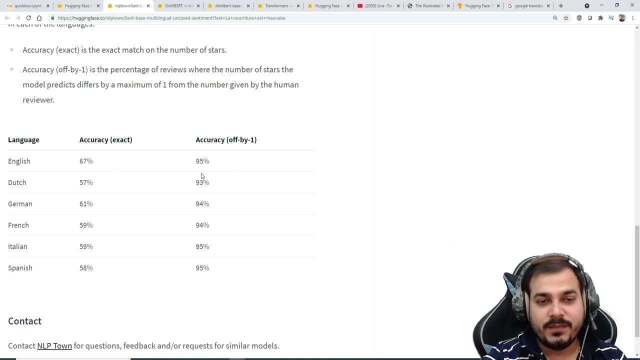 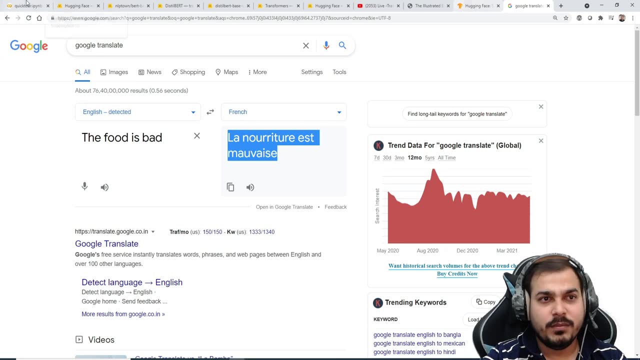 You can see 65, 67% exact off by one 95%. So these are some of the metrics they have performed and they're given the accuracy. Okay, Now let's try with something like: I hope this also supports This is also good because the right hand side 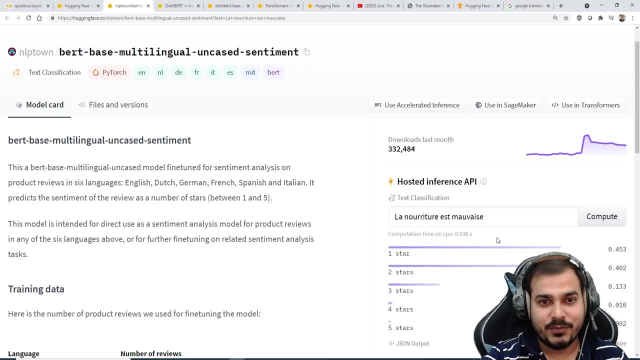 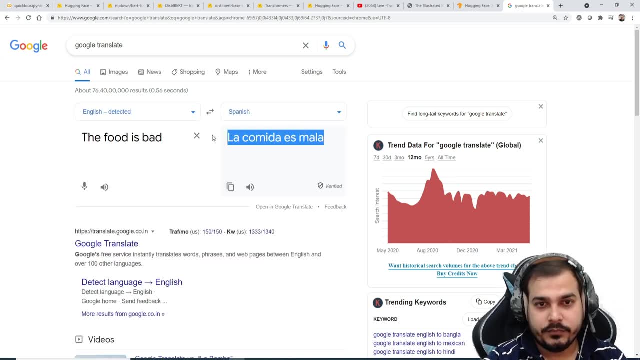 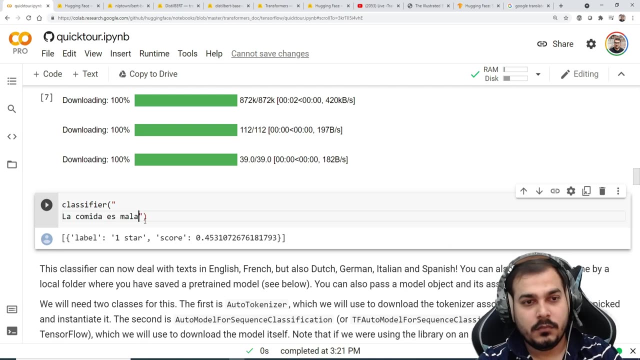 you can see the examples also, guys. Okay, And probably you can test which all things are there. Let's convert this into Spanish. Now I think Spanish is also supported. I'll copy this And probably I'll paste it over here and I'll paste it and execute it. 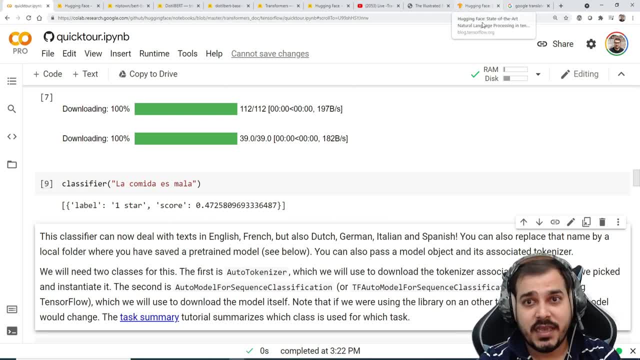 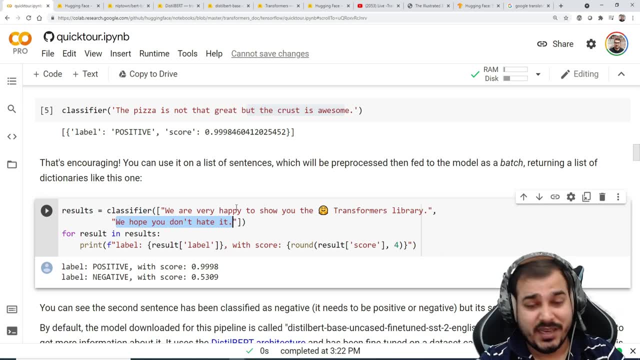 So again it is giving one star and almost the accuracy is same. Let me take the same example. We hope you don't hate it. I'm just going to copy this just to show you an example. Pretty much amazing. I love the work that a hugging face is actually doing. 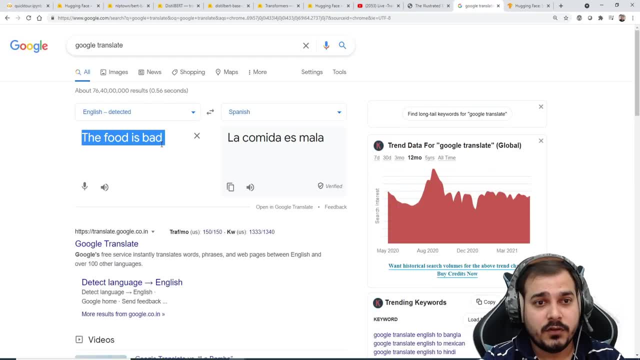 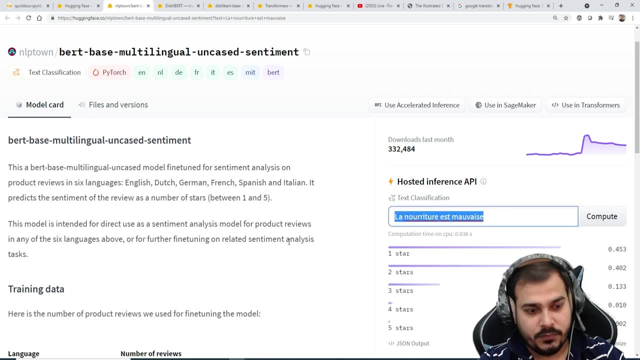 Okay, It's very, very good. It's very, very good, So I'm just going to copy It over here And now. this is my Spanish one. Okay, And let me test it over here first, If I execute it and compute it. 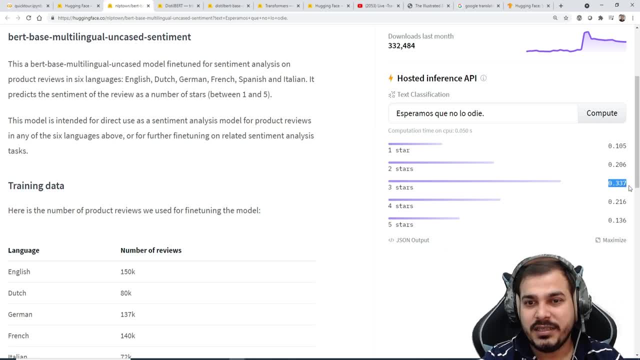 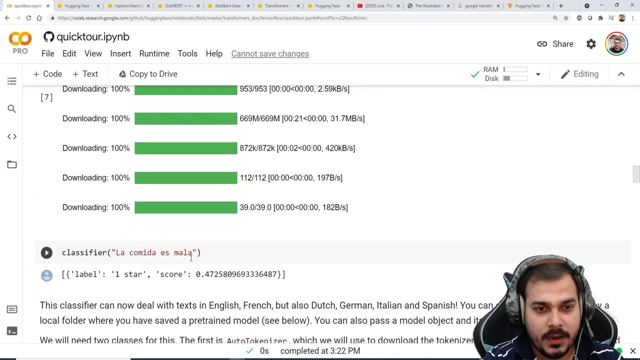 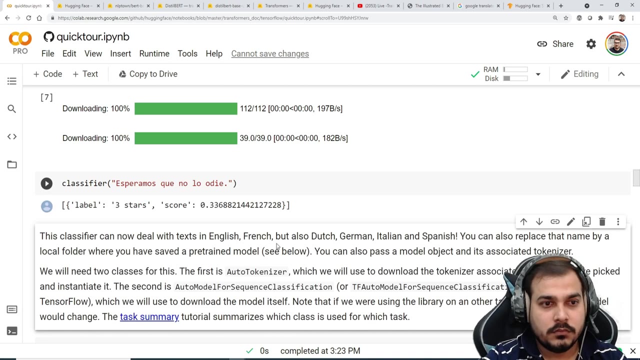 So here I'm probably getting three star as the highest point, three, three, seven. So here I can. I will be getting the same thing. I'll paste it over here, So here you can get the same output. Okay, So almost you're getting the same output. 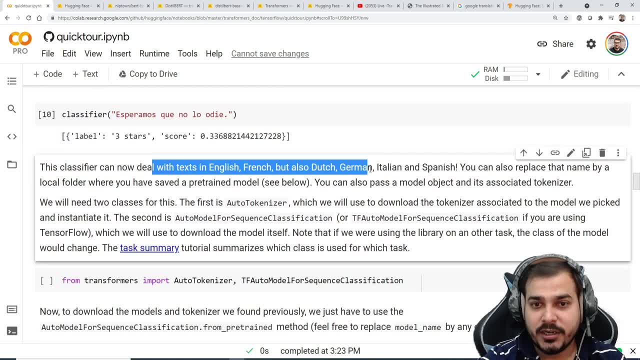 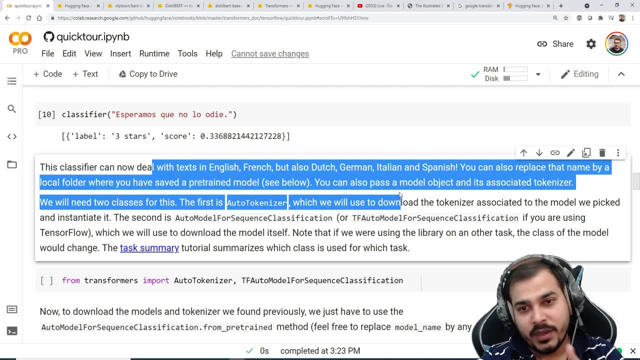 Okay, The classifier now deal with text in English, French, but also German, Italian and Spanish. You can also replace that name by a local folder where you have saved train model. Okay, You can also download the same train model, probably in a local folder, and you can also do it. 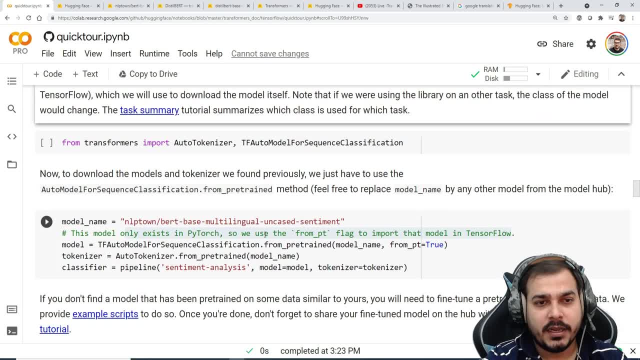 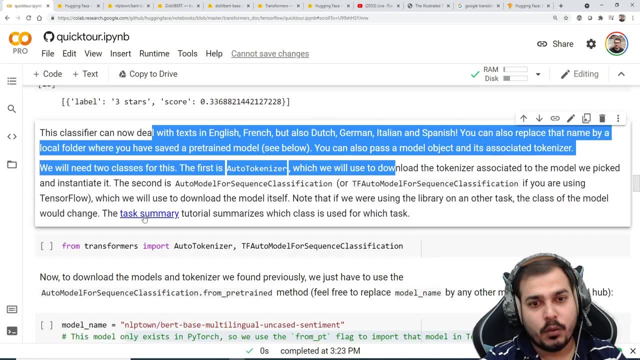 Okay, Now this is very much important, guys. Now we really need to understand what exactly is actually happening. Okay, And right now we have called like this: Now what if I want to call it to a local folder and probably do it? 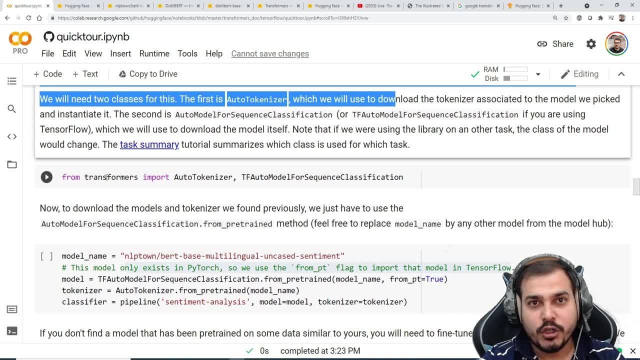 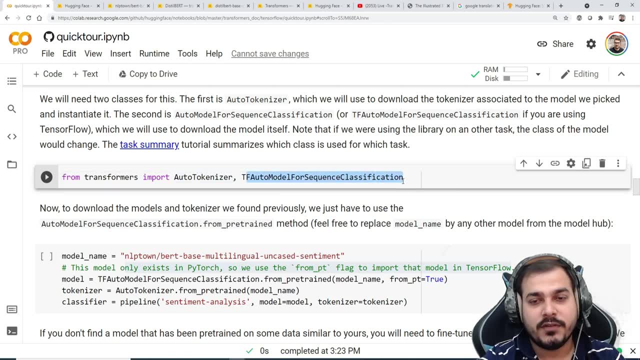 Okay, And for this the steps are something like this. So here I'm going to use tensorflow, So I have to use from transformers import auto tokenizer and TF order modal model for sequence classification. Now, very, very important information, guys: If you're working with this transformers of this hugging face. 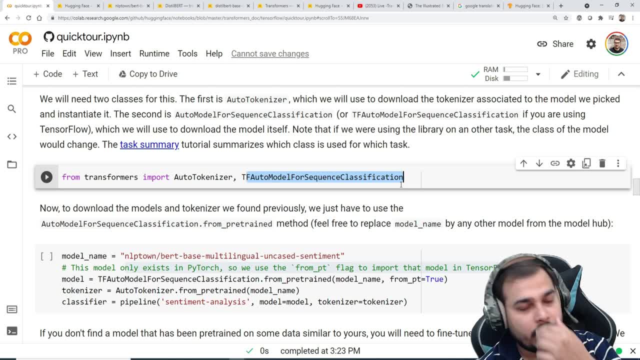 you know, always remember, whenever we call any kind of model, Okay, Probably you want to call it in our local and probably we need to fine tune, train it right. We have to usually go with this process what I'm actually going to show you. 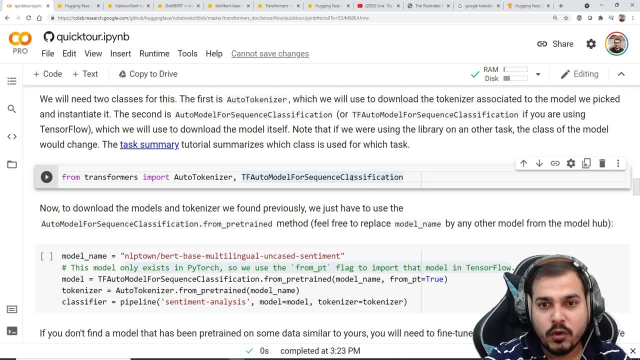 Okay, But remember one thing: whenever we need to call this particular model, we also need to call the tokenizer. See, there are two things that I'm being called with respect to this kind of NLP models. One is tokenizer- tokenizer. The role of the tokenizer will be that it will take the test data. 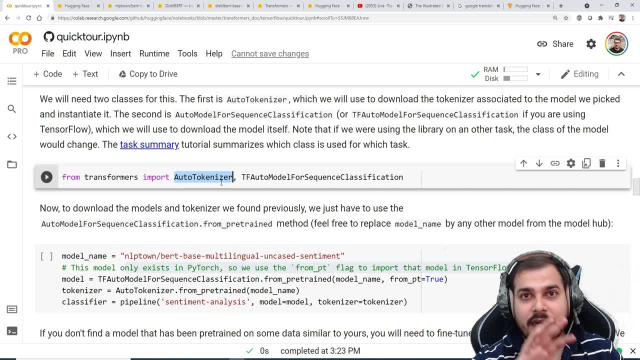 It will convert into some numerical data. Okay, It's just like how we use word embedding word to work, because text preprocessing is the most important task, And with respect to each and every algorithm, there is a different, different tokenizer. I'll talk about more in detail. 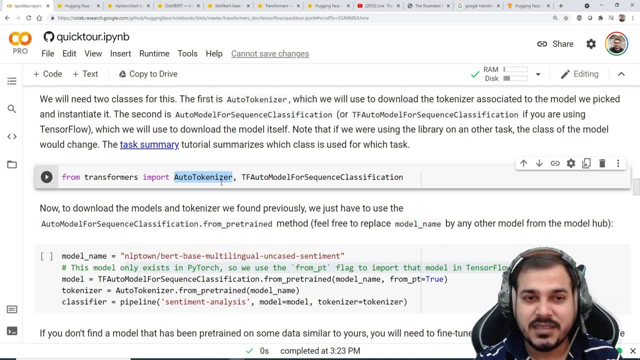 In depth, guys. there is a big, big different, different types of tokenizer. This is basically used. We'll discuss it: how each and every tokenizers work. Okay, And after we convert that, after we take the sentence and convert into a tokenizer, and then only this particular model will be able to classify it, 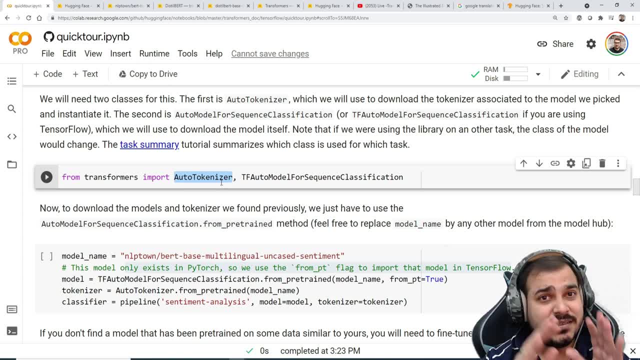 Okay, That is how it is basically trained. Okay, So tokenizing is the very much important thing with respect to anything that we do with respect to NLP. Okay, So here I will just try to execute it. So here I'm going to download one tokenizer, and one is TF. 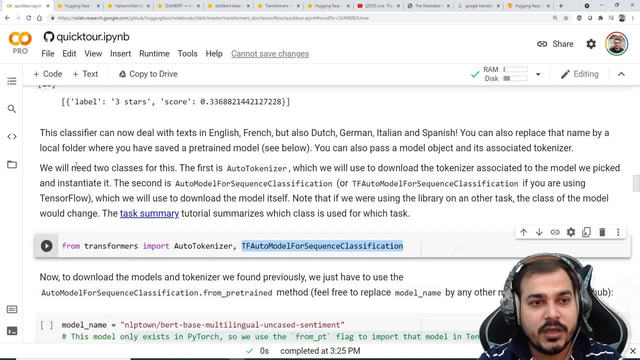 Model for sequence classification. Okay, Um, here you can see. we need two classes for this. The first is to auto tokenizer, which will be used to download the tokenizer associated to the model we picked and instantiated. The second is auto model for sequence classifier classification. 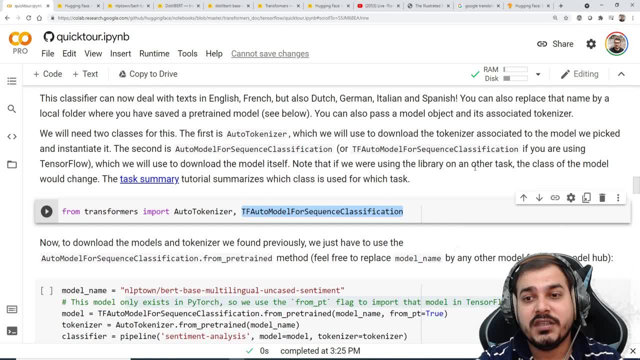 Okay, Which will be used to download a model itself. Note that if you are using the library on the other task, the class of the model would change right. So right now, this is a sequence class, if we can. text class, if we can. 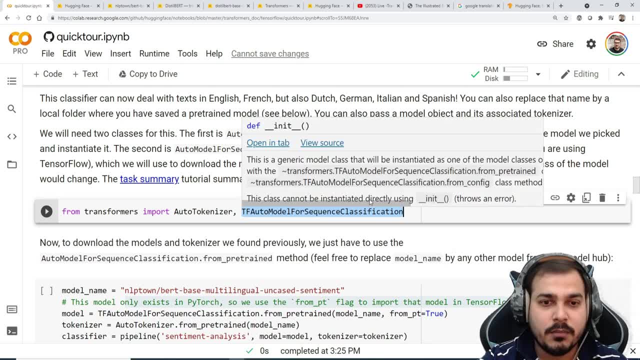 So I'm using this particular model. tomorrow I'll be doing a text, Okay, Text summarization. Again, the model will change. Okay, Now let's see how it is given. Now I've I've taken this NLP model. 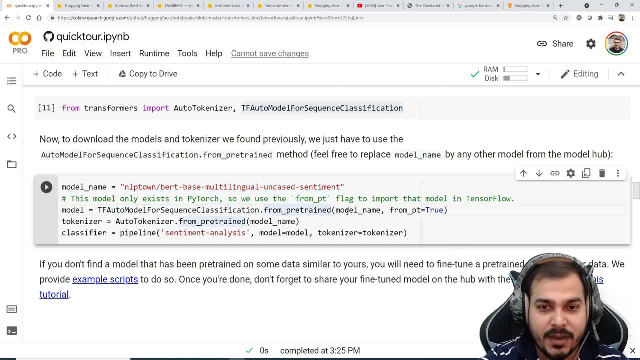 I'll use this NLP model for sequence classification from three trade model. I'll give the model name over here And remember guys, by default this model will be available in PyTorch. This model exists only in PyTorch So we can actually take it and we can import it to the model in TensorFlow. 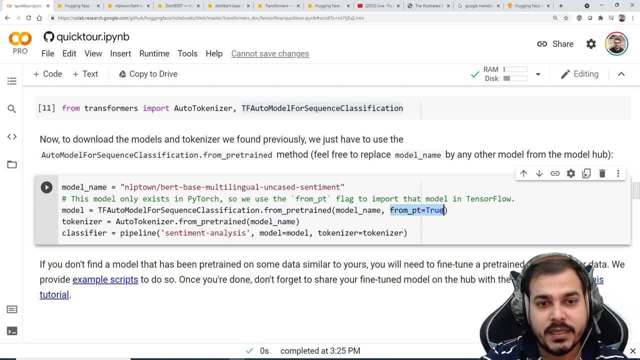 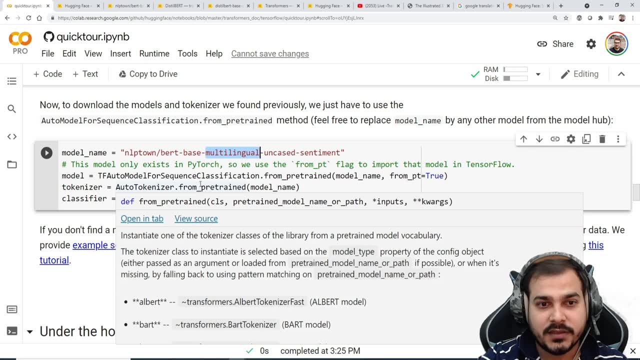 Okay, That is the comment return away. So we are giving from underscore: PT is equal to true, Then this auto tokenizer Based on this particular model. there will be a separate auto tokenizer, So we have to use auto tokenizer from pre-trained model with the model name. 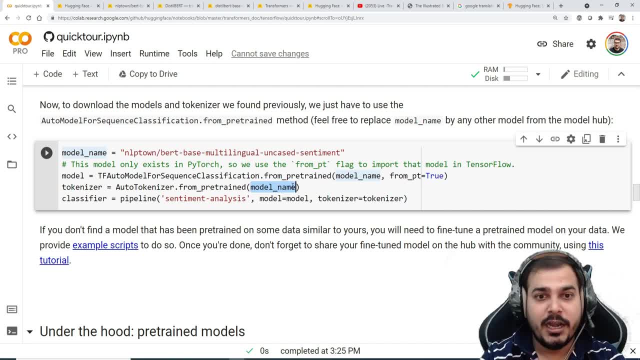 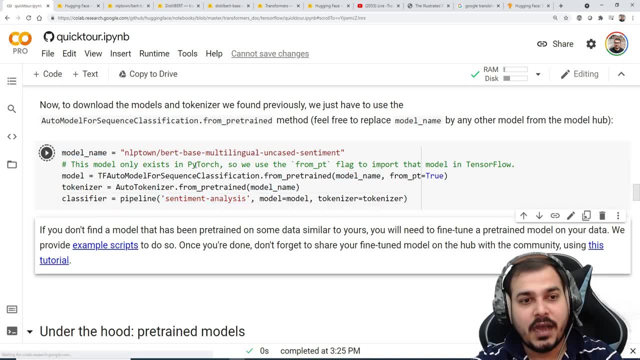 So, whatever is the tokenization process for that specific model, it'll get downloaded. And then, finally, I'm calling this pipeline sentiment analysis, model this and tokenize of this. This is how we do with respect to, uh, if you really want to do it in your local. 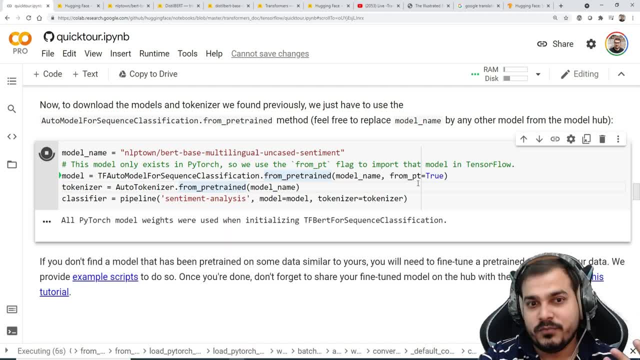 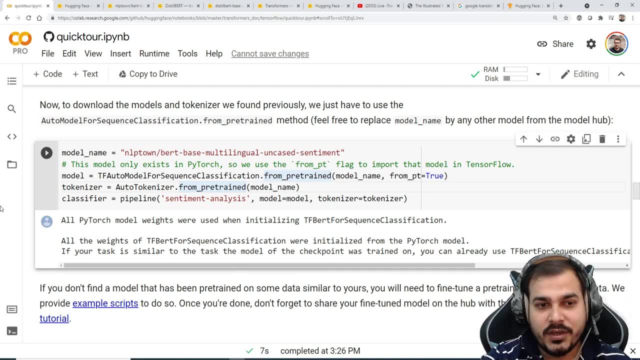 right. So first of all, it will download this. It will then, um, you know, it will then download the tokenizer. Then we have to call the class, The classifier. Okay, So here you can see all the weights for this volume. 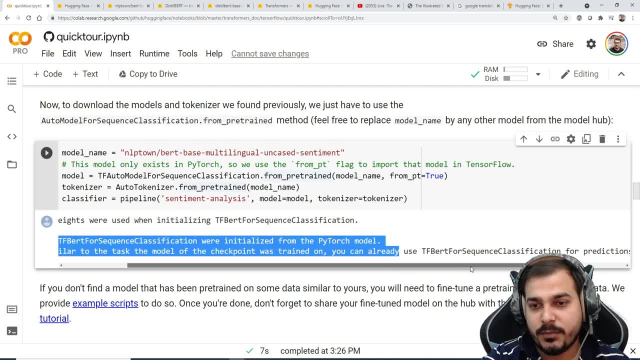 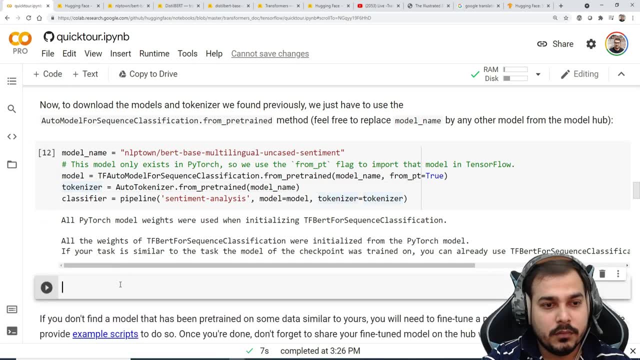 If I initialize for not by touch model, if a task is similar to a task, the more checkpoint was trained, then you can use this particular thing for production without future. Now you can do the same task wherein you've just give a classifier, and here I am a good boy. 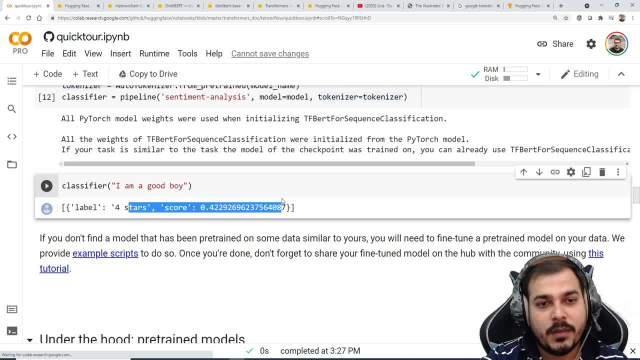 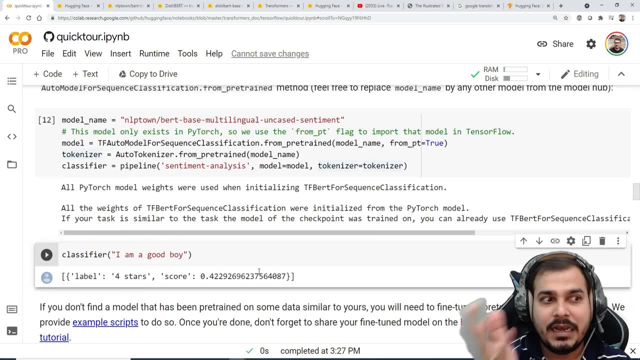 Okay, So here you can see that I'm getting the accuracy with level four, level four. basically It means yes, I'm getting a very good accuracy in shot. Okay, Label which is greater than label three. At least it is positive what I see. 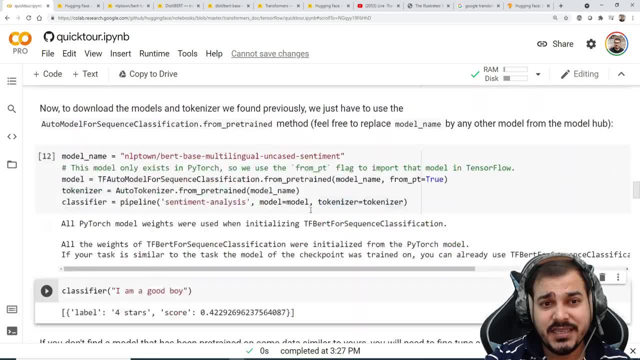 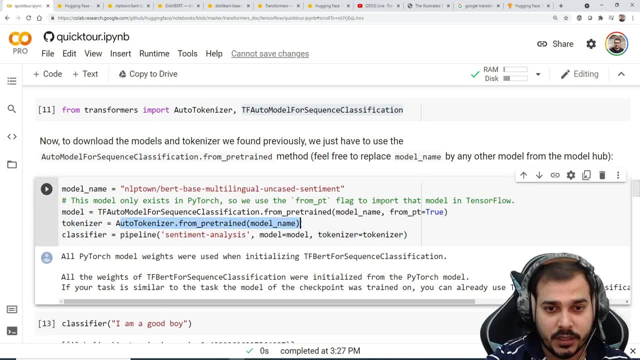 Okay, So I hope you have understood this, guys. We will be seeing a lot of things, Okay Now. okay, Let me just make you understand how this tokenizer also work. Okay, Now for this particular task under the hood. let's see how it works. 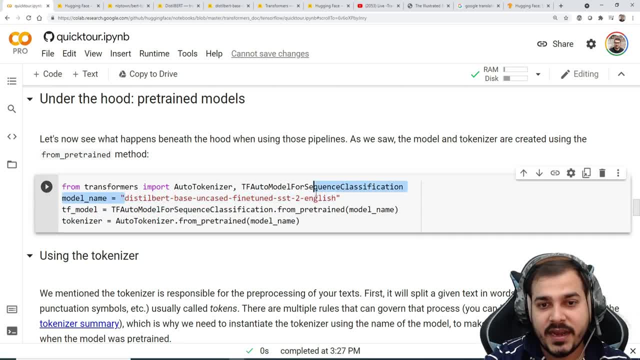 Now suppose I'm using this particular model- distilled but uncased find, assisted to English- And I have downloaded this model and I have downloaded the tokenizer. Okay, So tokenizer. I hope everybody's understood why this is downloaded. Now let's use this particular tokenizer and remember they are different. 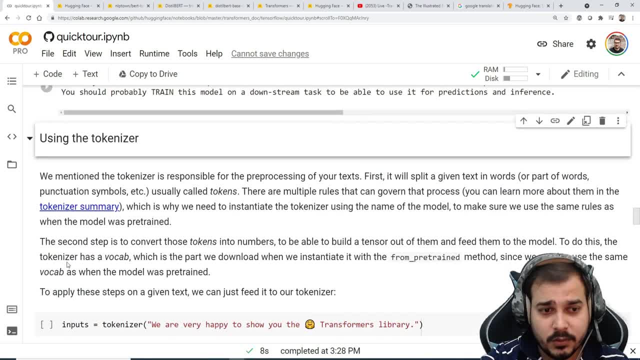 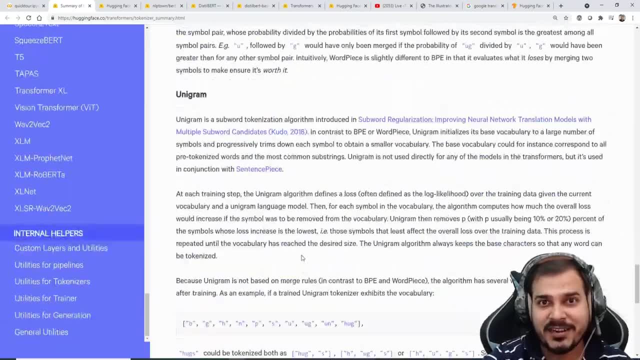 different tokenizing process guys. Okay, Um, there's a good, amazing tokenizer summary page. This many different types of tokenization are there. This you really need to read and understand. but I will teach you everything, Don't worry. 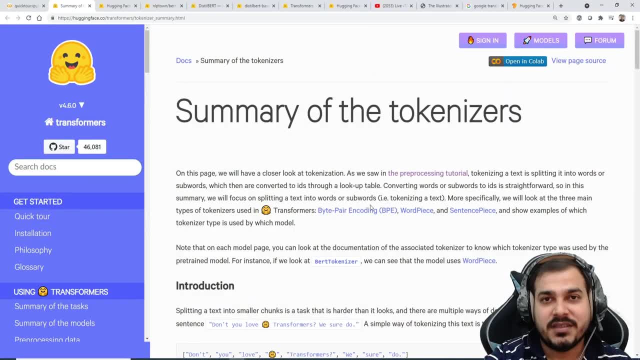 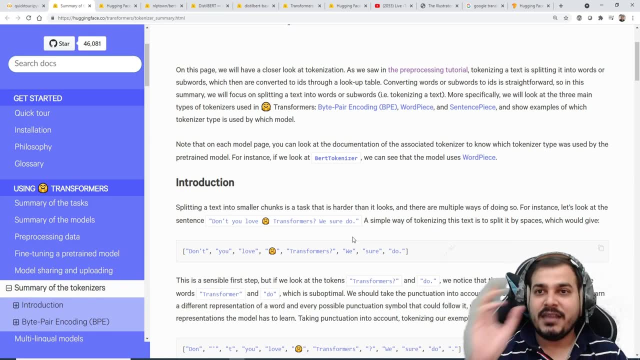 Whatever things are there, what this? the documentation is pretty much amazing. Again, I'm telling you of the hugging face. We'll try to understand tokenization process. Two main things in hugging face is tokenize yourself, And then the model architecture. 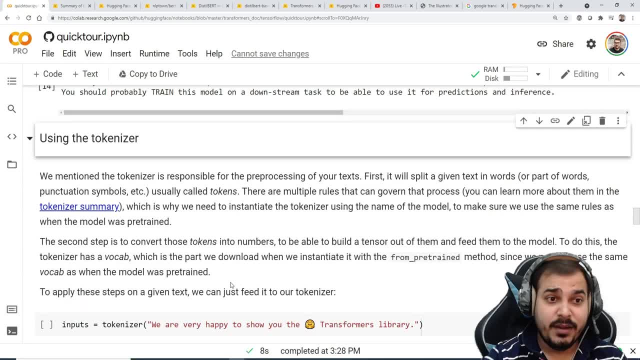 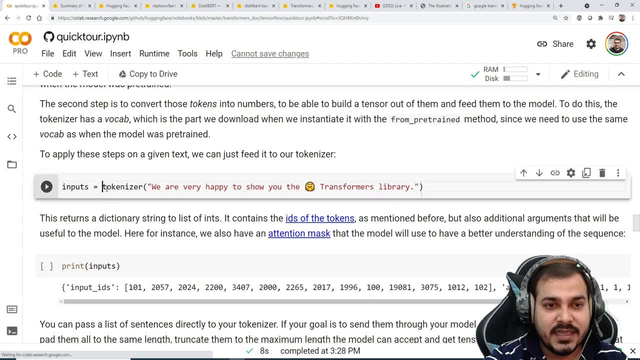 what it is basically doing, because that specific model is trained by using this tokenization process. Now this is downloaded. Okay, Now let's see one step. Suppose if I take this tokenizer. this tokenizer is nothing, but this is initialized from auto tokenizer, from that pre-trained model. 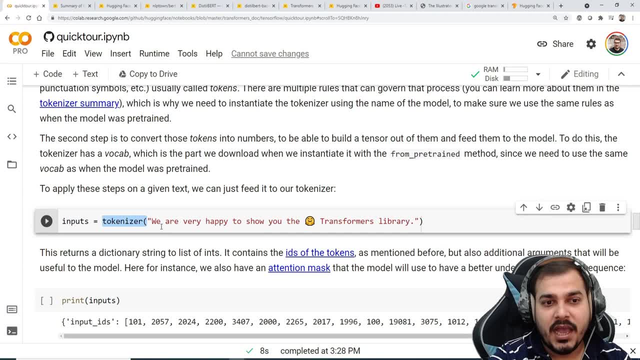 which is given as a model name. over here I have my tokenizer variable. I'm just writing. We are happy to show you the the transform our library. Now let's see how this entire word is converted into a tokens. Okay, So I will make a code, and now here it is. print of inputs. 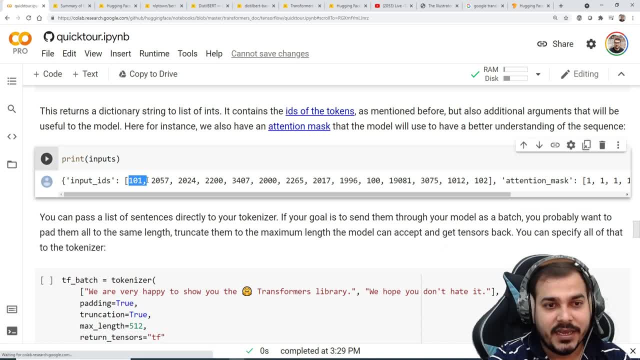 If I input this here, you can see that every input ID, every word, is basically given by a numerical number. Okay, This numerical number is basically treated as IDs of the tokens. Okay, These are basically the IDs of the tokens, like how we do it in word to bank. 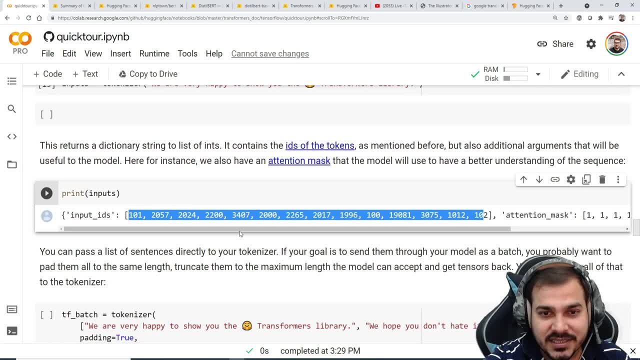 We provide Some numerical values, probably some indexes. Similarly, this does that same work. Yes, Remember, right now, by default, this particular tokenizer is fixed. right, I may also change this tokenizer length in order to change. Probably I'll be using something like this tokenizer. 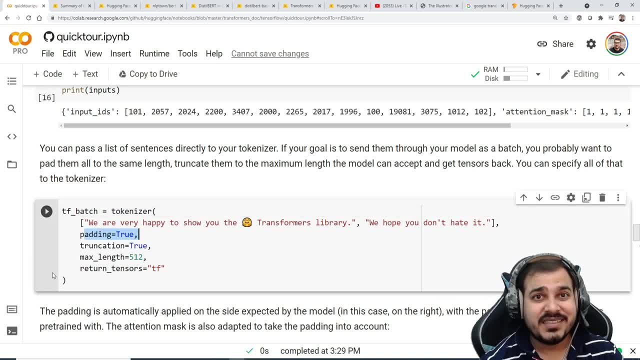 Padding is true. Padding white is required to make all the sentences equal right. That is why padding is required. Then truncation is equal to true. If any spaces are there, that will get removed. Max underscore length is five, 12.. 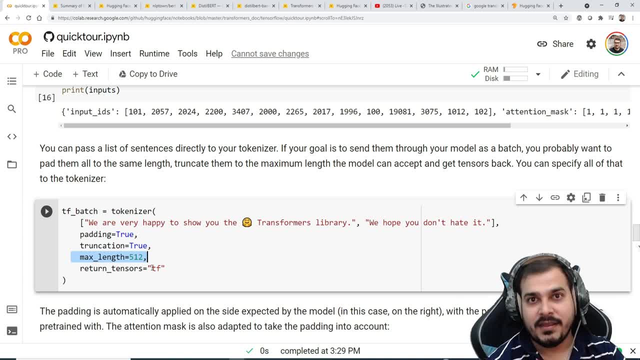 So here I'm saying that every uh, the maximum length for a particular sentence will be five, 12.. Okay, The maximum length that we can take in this sentence is five, 12. Okay, So once I execute and see my TF underscore, batch here. 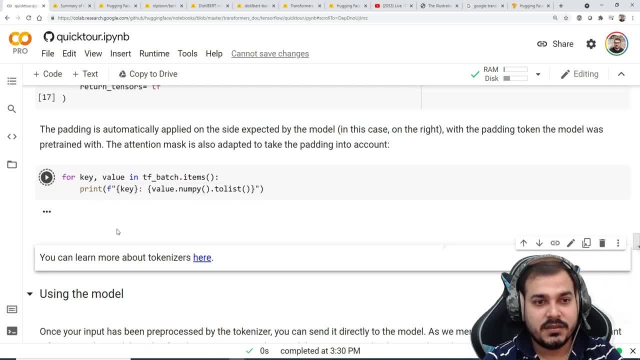 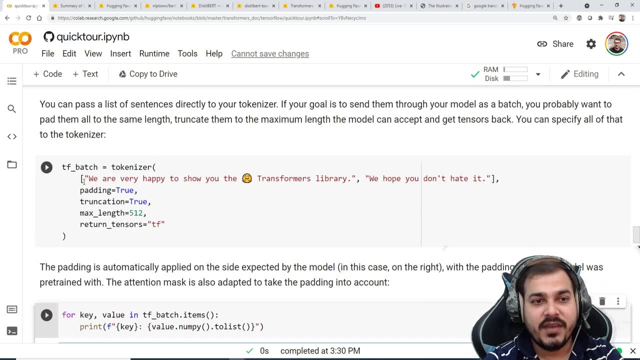 you'll be able to see this. So if I execute this here, you'll be able to see this guy. See, everything is shown over here, right? Pretty much easy, Pretty much simple. here We have given two sentences. This is one sentence.